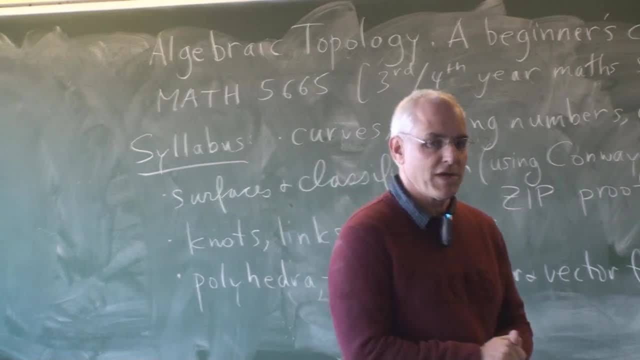 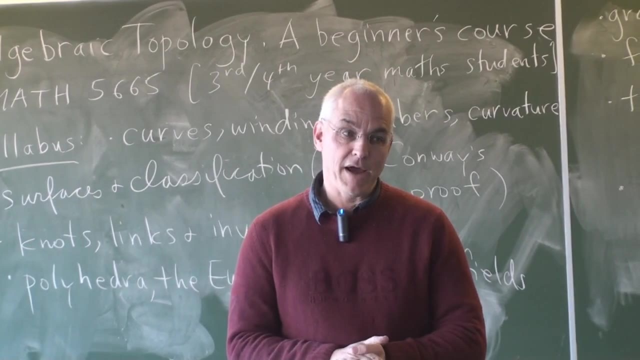 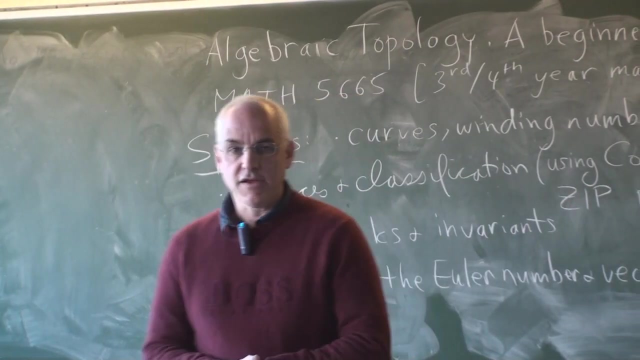 which developed from 19th century work in complex function theory, due to Riemann primarily, and then taken up by Henri Poincaré, a great French mathematician of the turn of the century, And he established a lot of the foundational ideas and further directions for the subject. 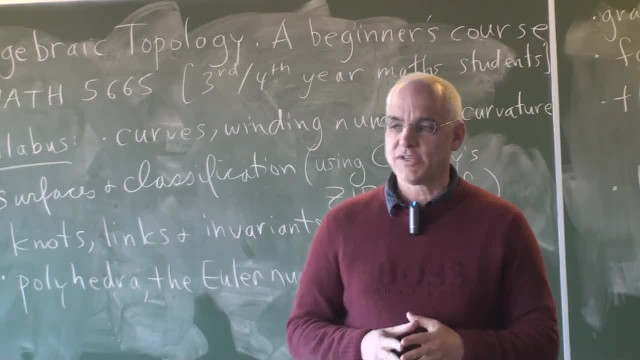 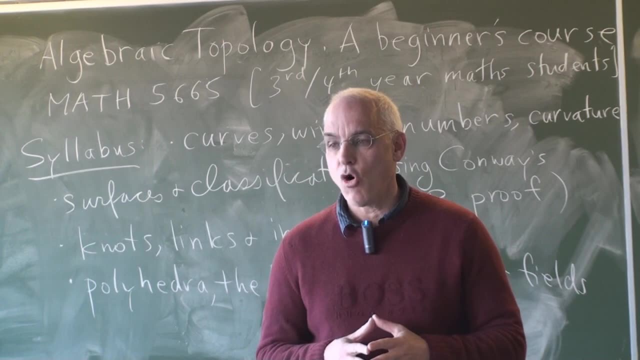 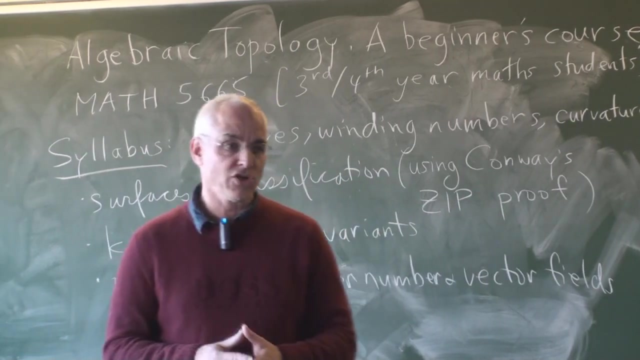 And a sense of the vibrancy of the subject is in the fact that over the last few years, one of the main open problems in this subject, which is also being considered one of the main open problems in all of mathematics, was solved, And it was called Poincaré's Conjecture. 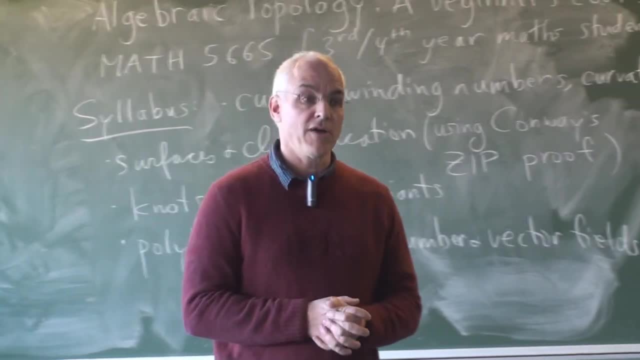 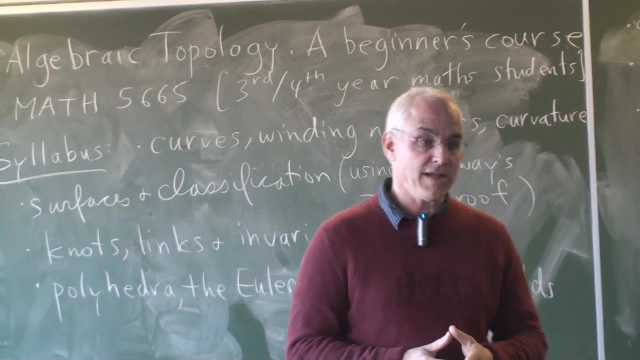 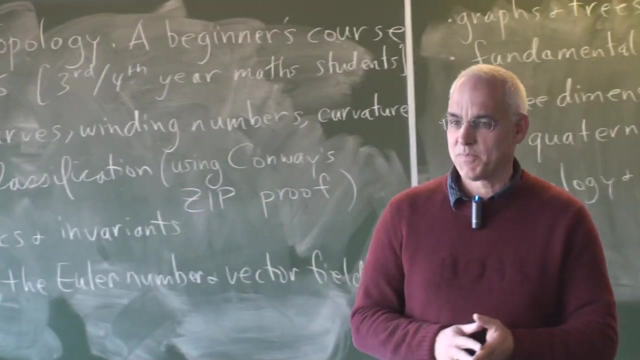 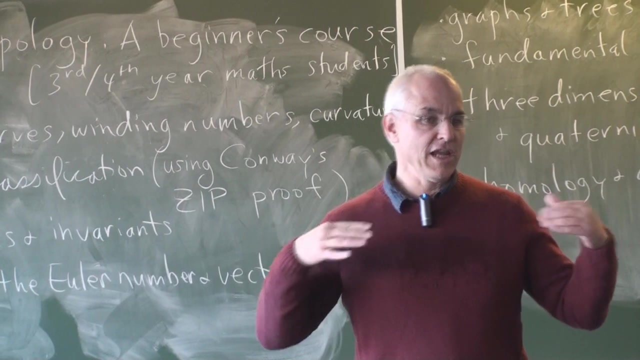 It was solved by a rather unorthodox and highly original Russian mathematician. You may have heard about that, So that's part of the story that eventually we'll make some contact with. Algebraic Topology is roughly the study of shapes- Shapes where we are interested in what is maintained when we continuously deform shapes. 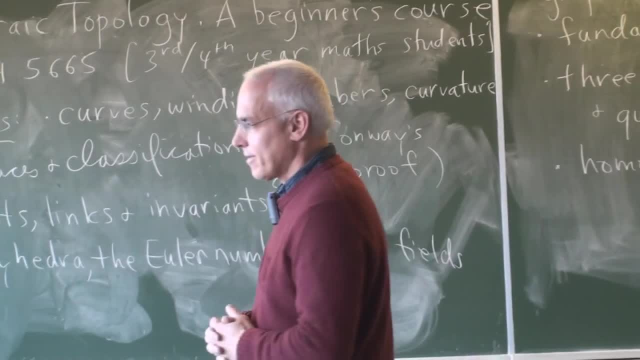 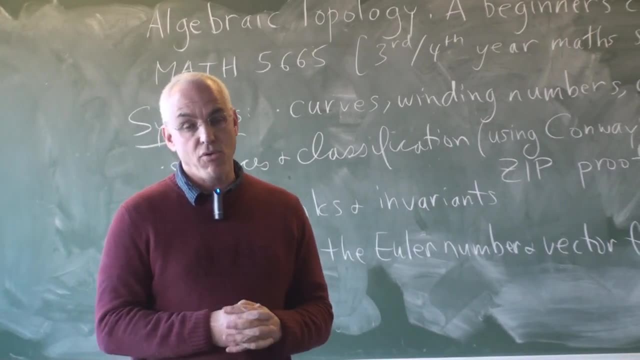 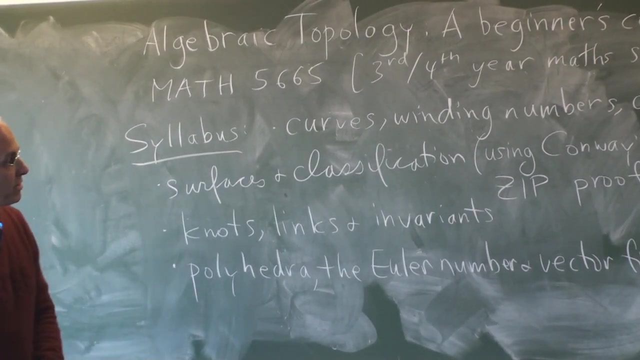 And it's got natural connections with differential geometry and with algebraic geometry and with modern physics. It's very important for modern physics. So this course is going to be touching base with a number of topics and I've listed them here. 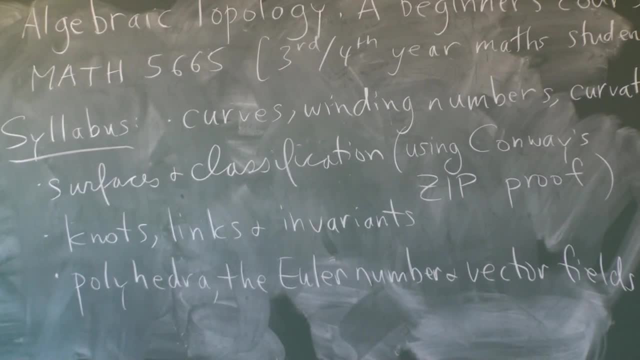 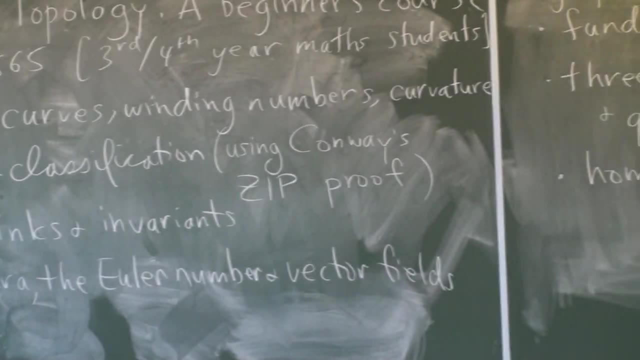 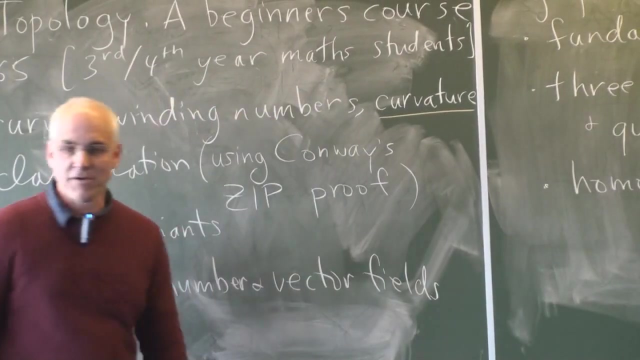 So let's just quickly give you an idea of where we're going to be going. So we're going to talk about curves, winding numbers and curvature, And one of the novelties of this presentation will be curvature. We're going to have a sort of a new way of thinking. 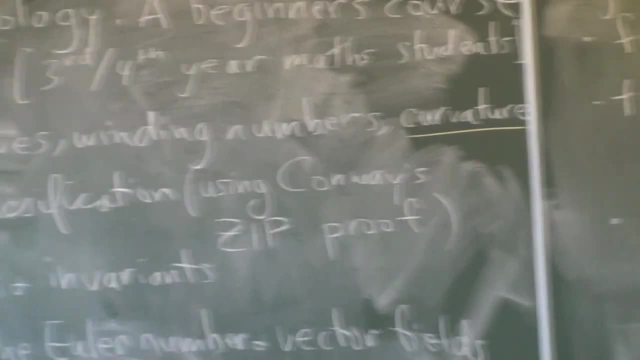 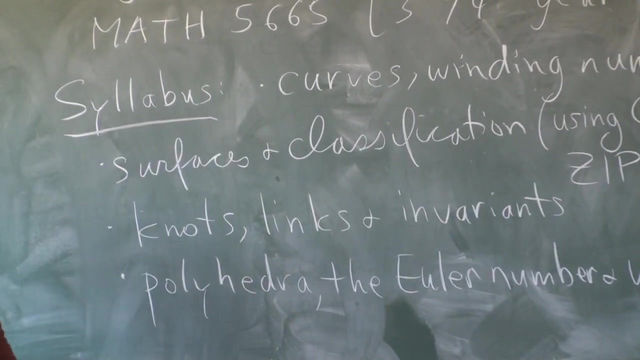 or somewhat new way of thinking about curvature in a very rational way. So that's going to be one of the novelties of this course. Another novelty is when we get to a very standard aspect, the classification of surfaces. we're going to use John Conway's Zip Proof. 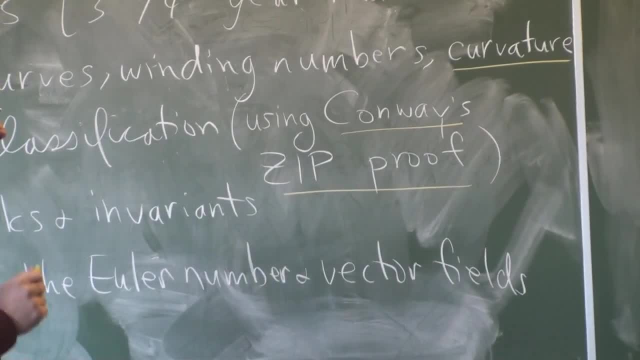 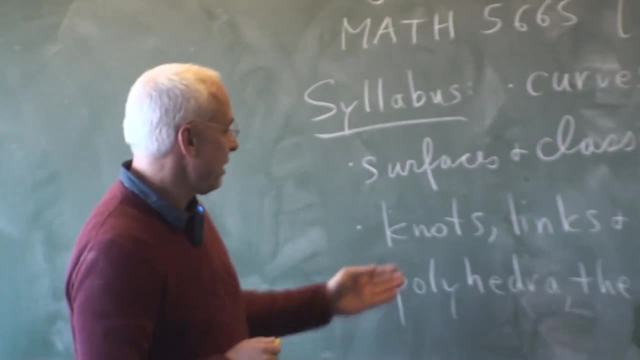 Which is? I don't think it's found in any of the texts on the subject. maybe some recent texts have it, but it's a very pleasant and insightful proof. We'll talk a little bit about knots and links and invariants of those. 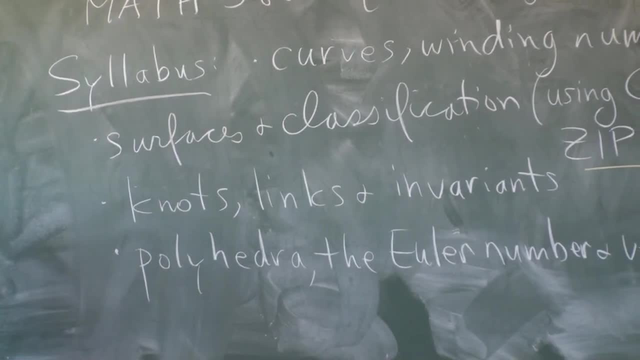 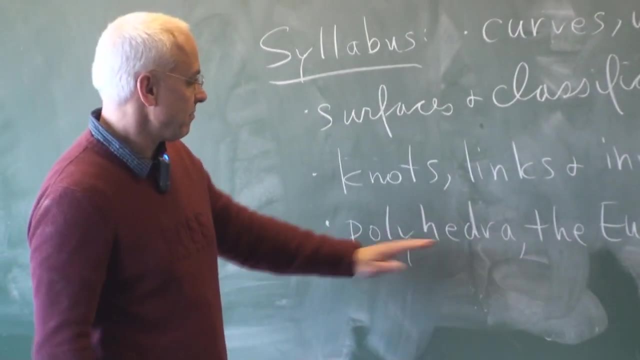 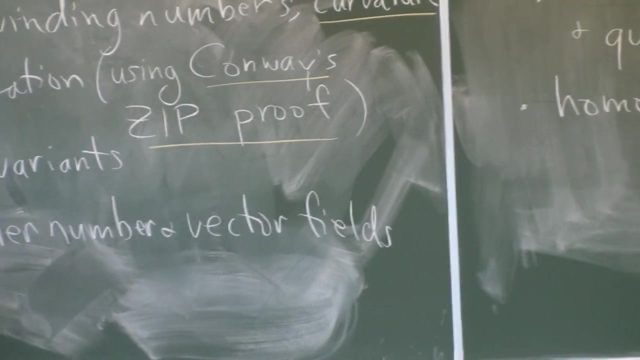 There are many invariants, but we'll just treat some simple ones. Then we're going to go back to a subject which is much earlier historically: polyhedra, the Euler number and vector fields. We're going to make some contact with graph theory. 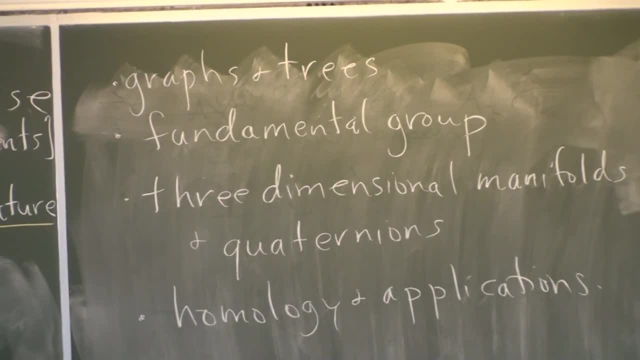 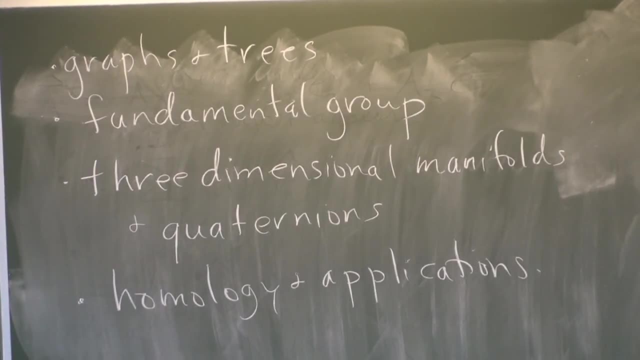 the topological aspects of graph theory and talk about trees. We're going to talk about the fundamental group of a surface or a topological space, which was introduced by Poincaré, And then we'll eventually get to talking about three-dimensional manifolds. 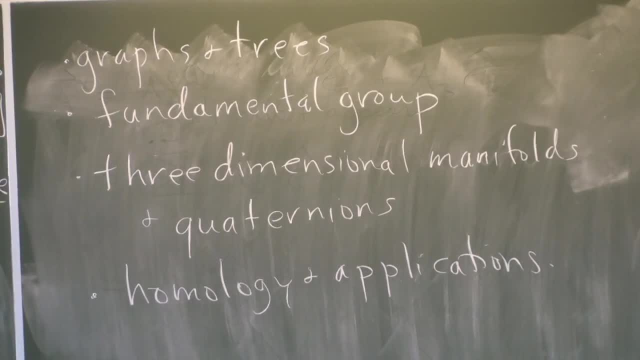 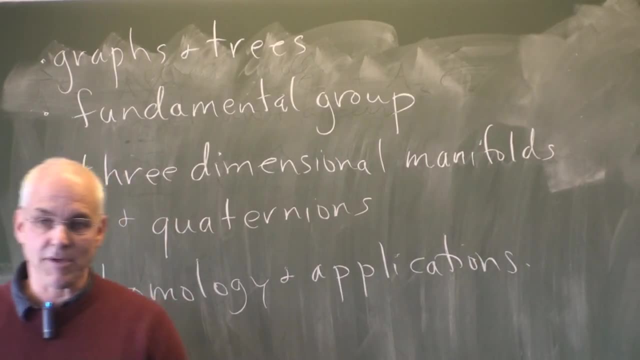 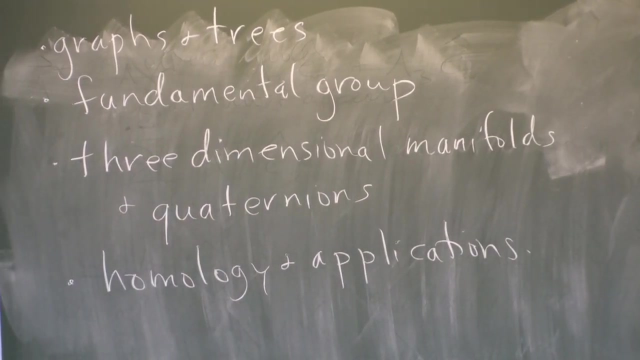 We'll take the step up from two-dimensional surfaces to three-dimensional manifolds, which is much harder, But we're going to have a good look at the most fundamental three-dimensional manifold, which is the three-sphere. It's a very rich object of study and naturally connected with quaternions. 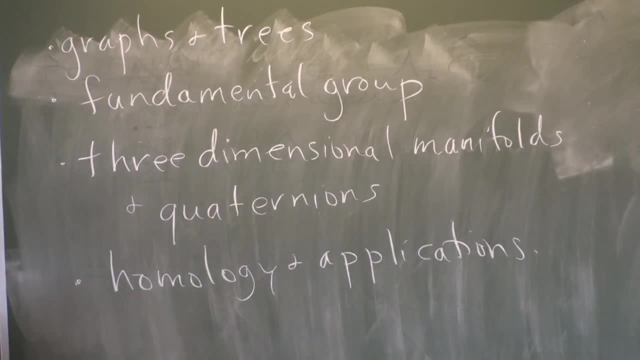 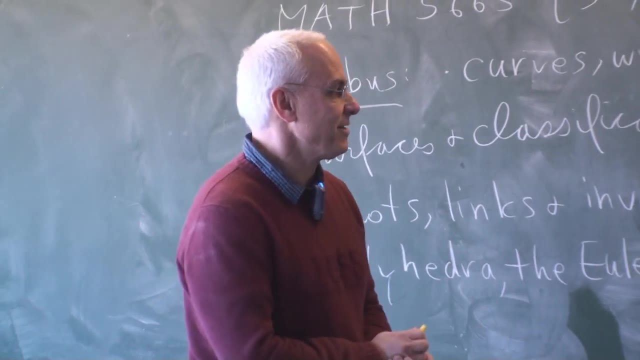 And then we're going to also hopefully talk a little bit about homology and applications. So some of these words will not mean anything to you, that's alright. But at the end of the course you should know what most of these words mean. 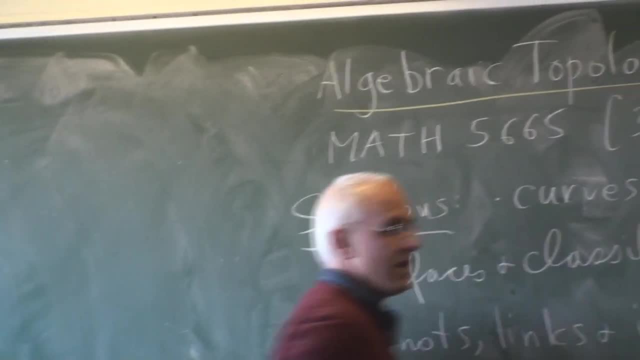 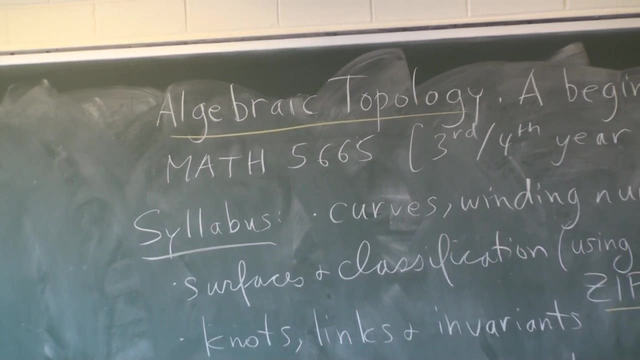 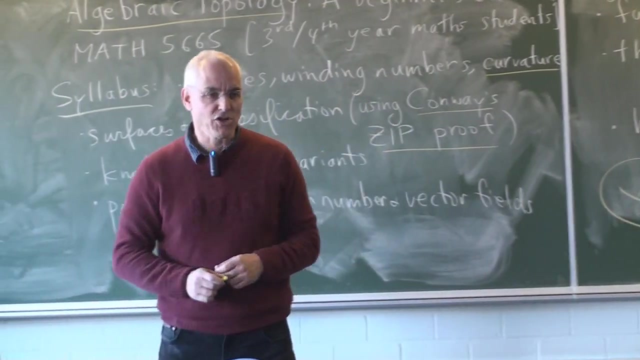 Now it's algebraic topology, So that means that algebra is used to study topology. We're interested in shapes, And a very common kind of shape is a donut- A donut shape, And this may not look exactly like a donut. 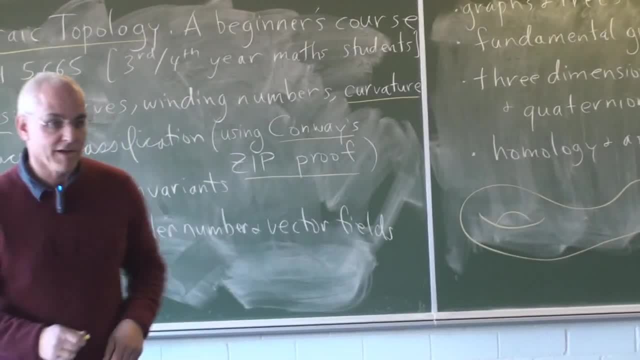 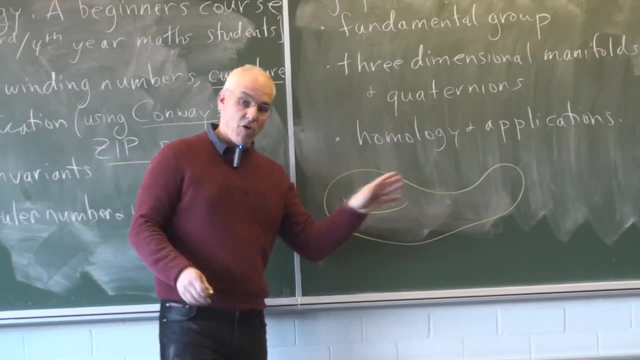 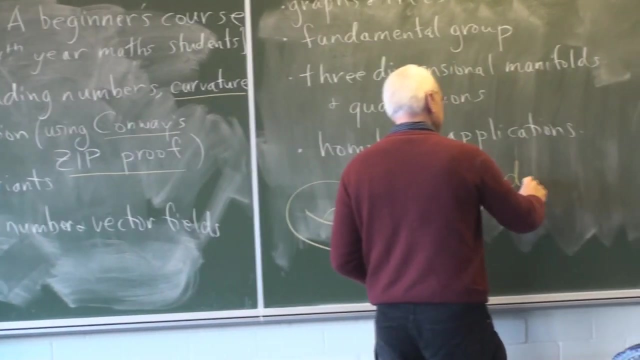 If this was served to you at Dunkin' Donuts you'd probably be a little bit suspicious. But in topology we're allowed to deform objects, And as long as we deform them continuously, we agree that they are the same. So this is a donut. 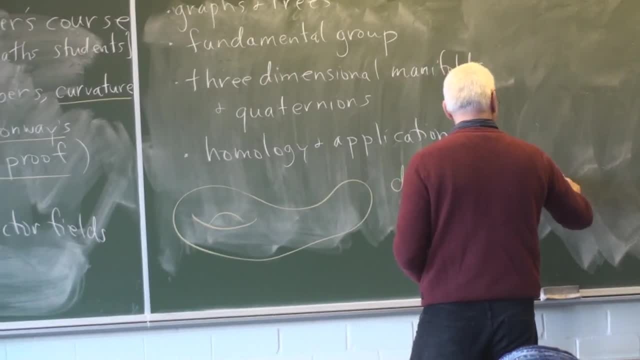 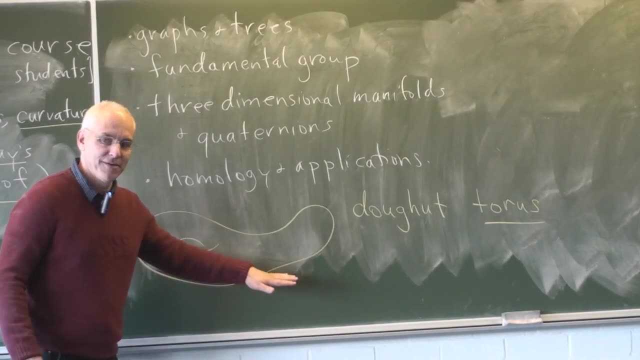 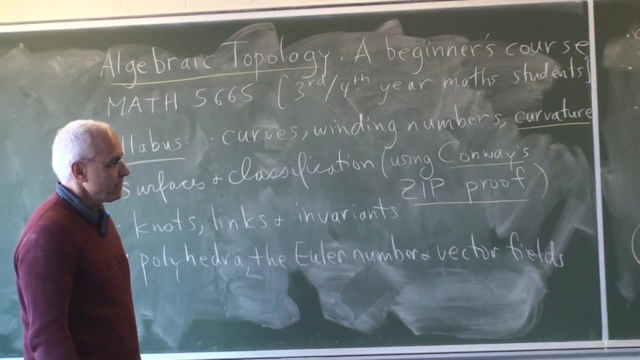 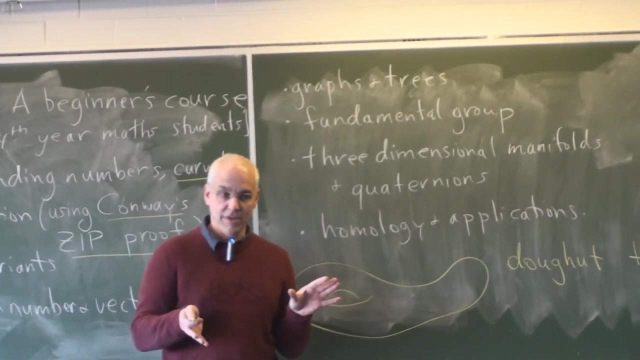 Or the mathematical word, is a torus, And from the topological point of view, it doesn't matter if we bend it, distort it, twist it. One of the ideas, then, is: although we're studying something which is very physical and spatial, 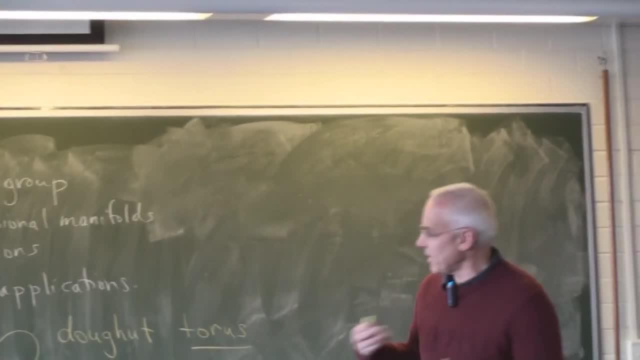 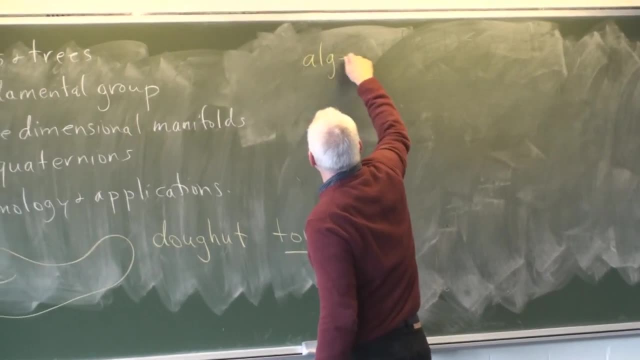 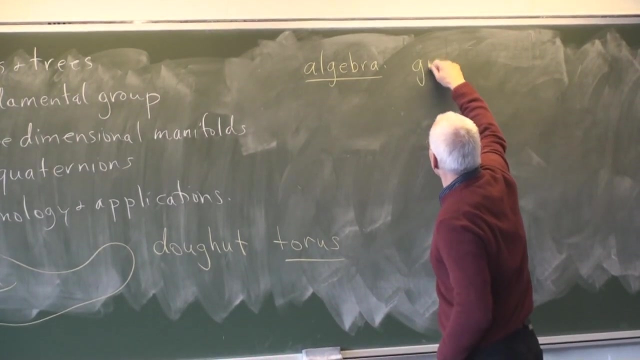 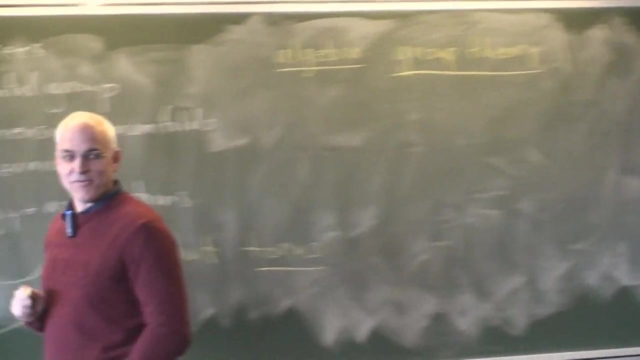 and we can make models of these things. we're going to be studying them from an algebraic point of view often, And the algebra that we're going to use is a branch of algebra primarily called group theory. Okay, so let me just ask you. 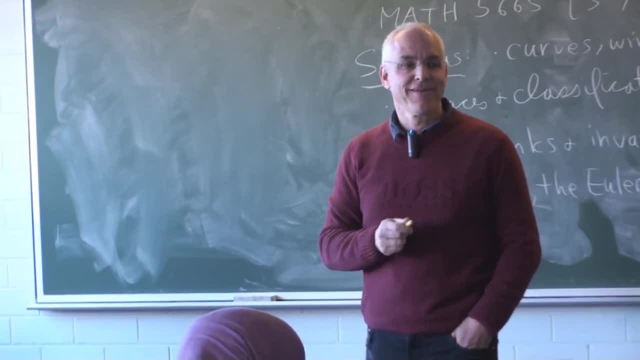 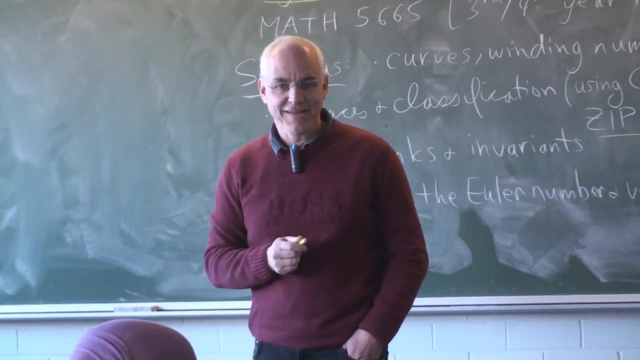 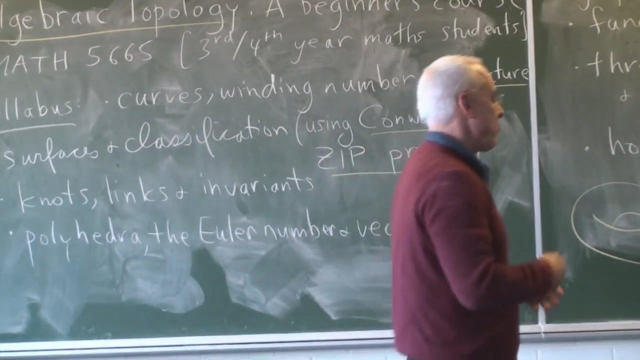 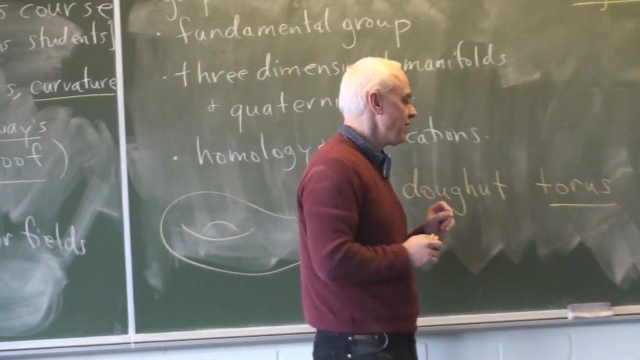 how many of you have taken group theory before? How many of you have not Not taken group theory? Okay, so we are going to use some group theory, but I am going to remind you and develop more or less the essentials of the group theory that we need. 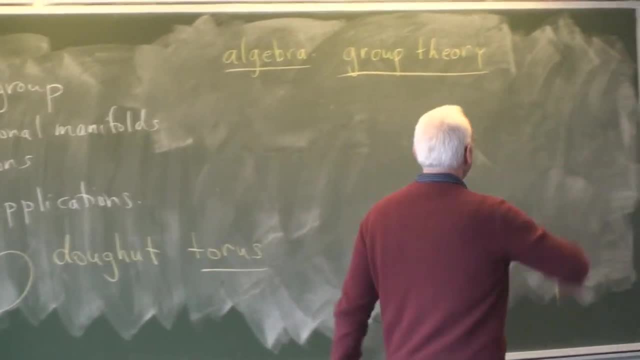 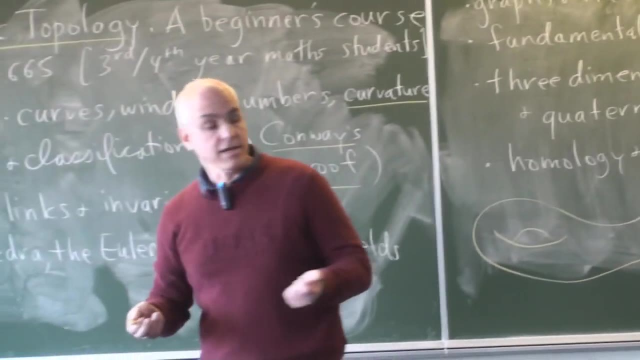 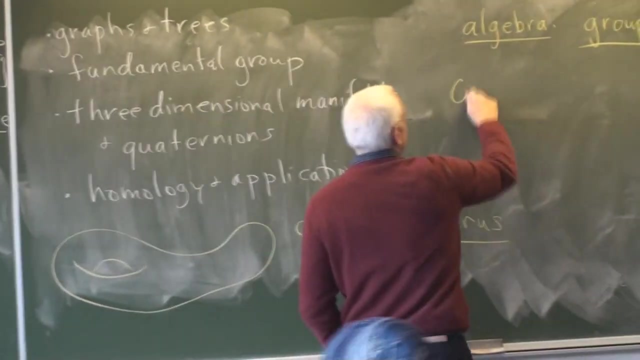 But nevertheless, it's a good idea for you, if you are not familiar with group theory, to brush up on that subject. That's going to be our main algebraic tool to study topology. Alright, so let's say what is algebraic topology? 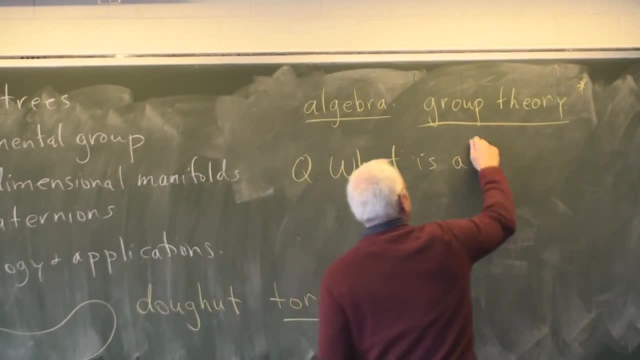 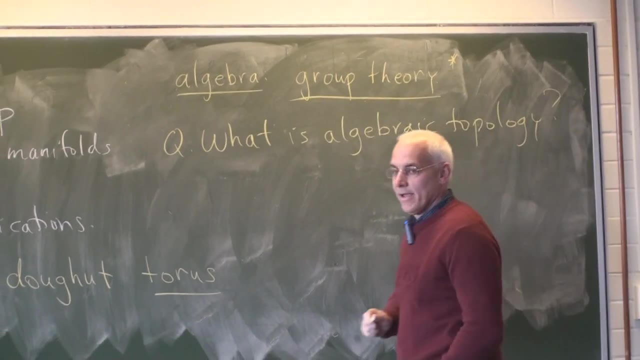 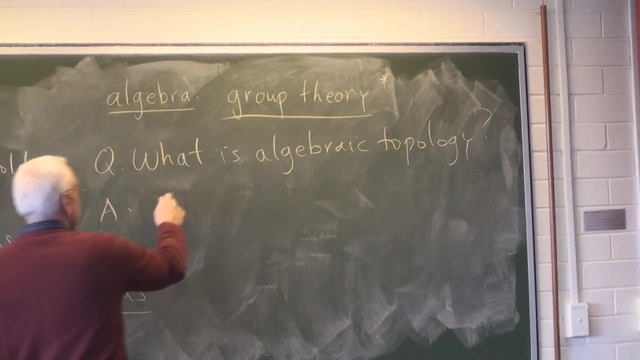 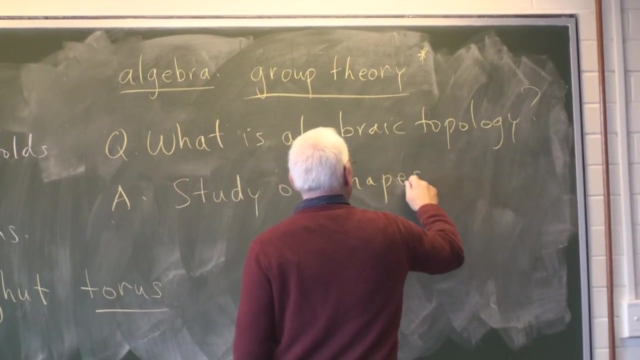 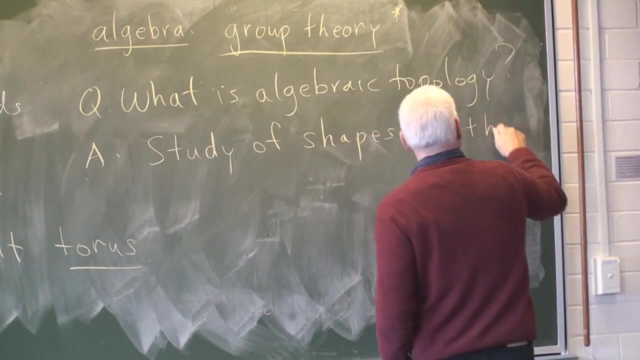 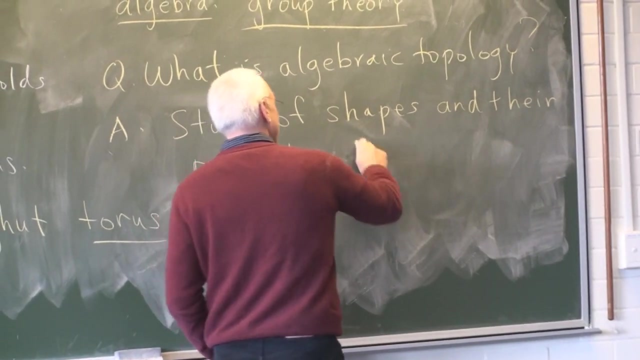 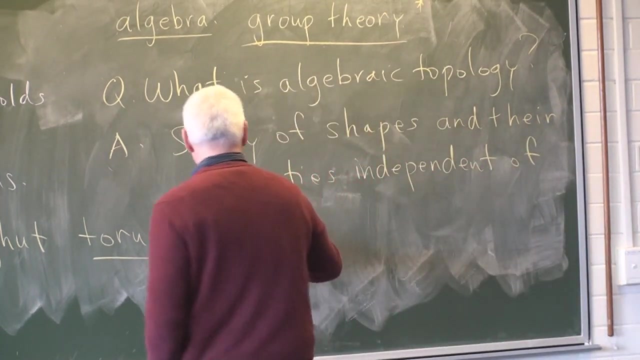 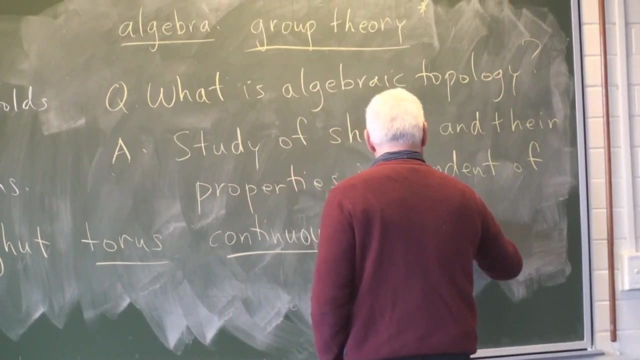 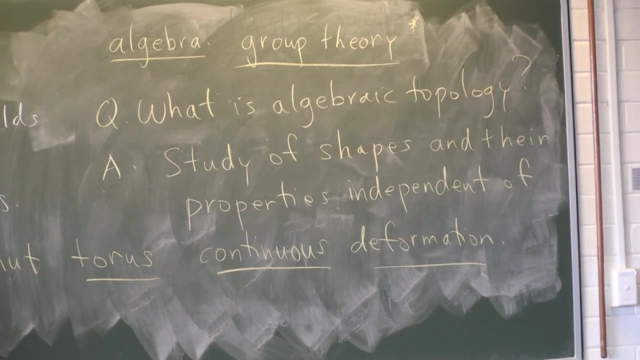 It's a natural question And I guess a first answer might be that it's the study of shapes, The study of shapes and their properties, and their properties which are independent of continuous deformation. So, for example, if we took this two-dimensional doughnut, 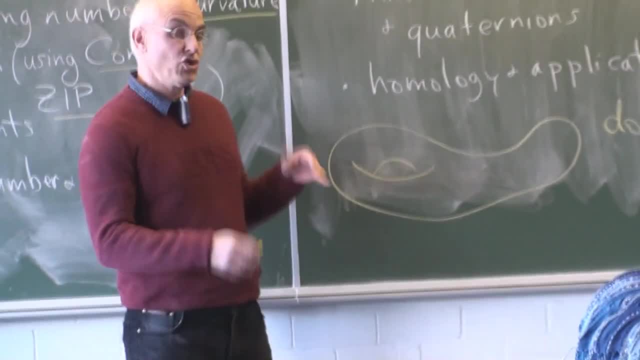 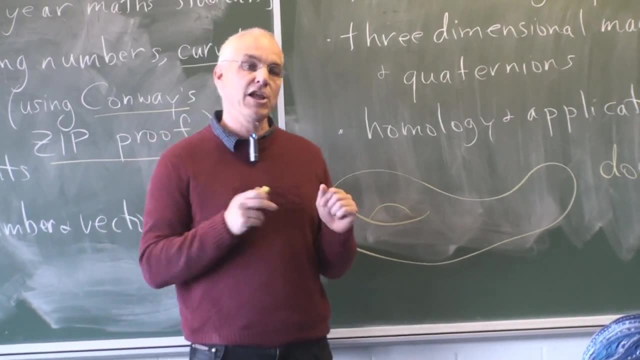 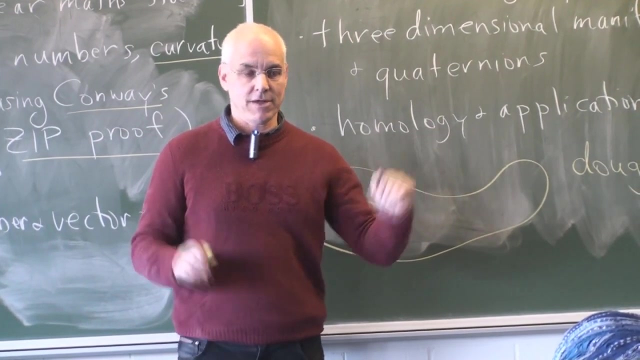 and when we think of this surface, we are thinking of it as a two-dimensional object. That means we are thinking of its skin as being the object of study. It's not the interior that counts, it's only the surface itself, And we can think of the surface as almost being made out of plastic. 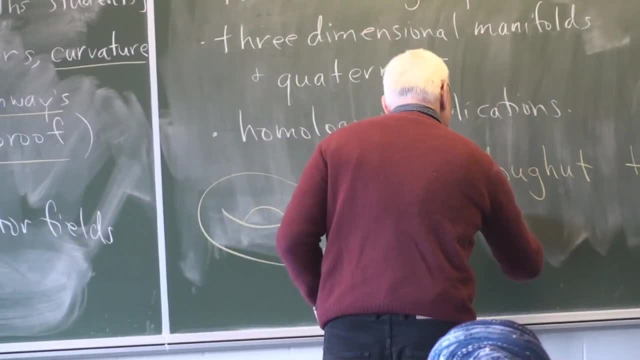 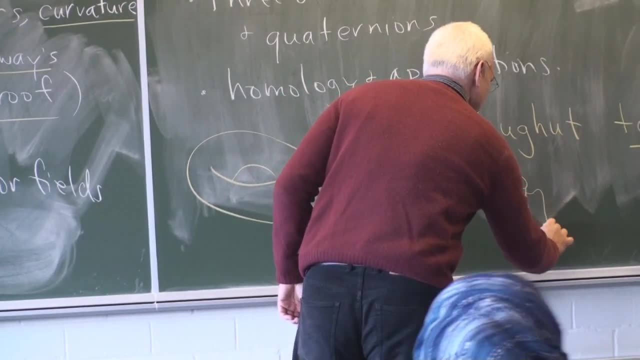 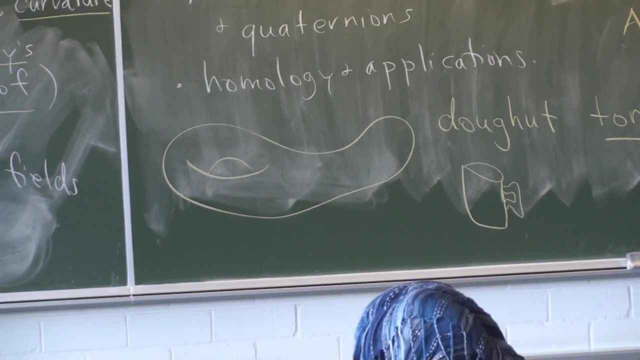 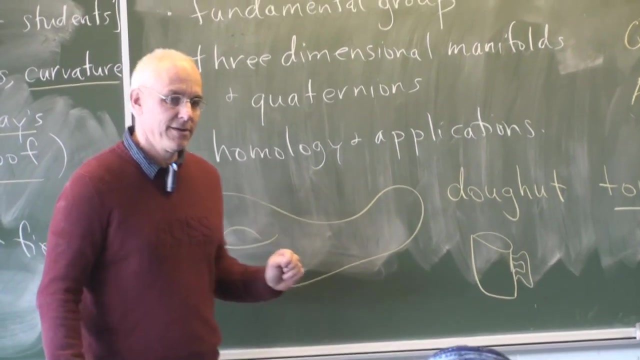 And you are allowed to deform it. and one thing that you are allowed to deform it into is a coffee cup or mug, And it's kind of a standard way of thinking to be able to see that the doughnut or the torus is really the same. 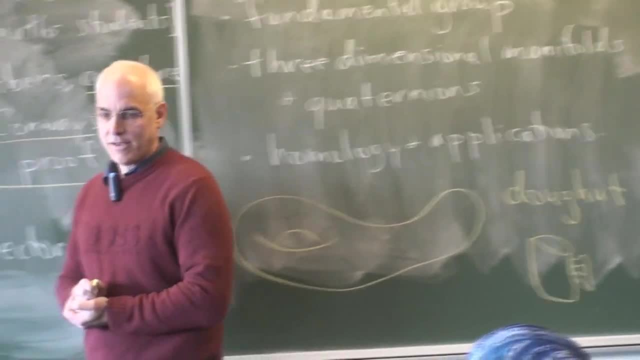 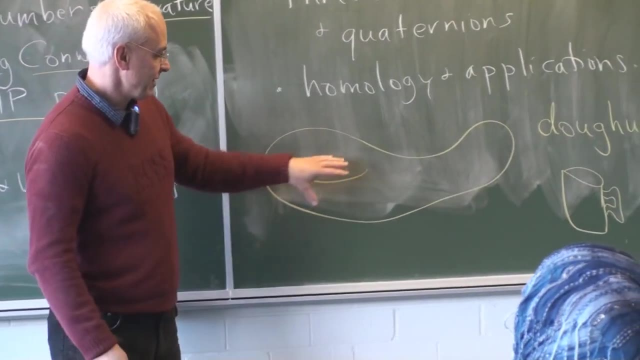 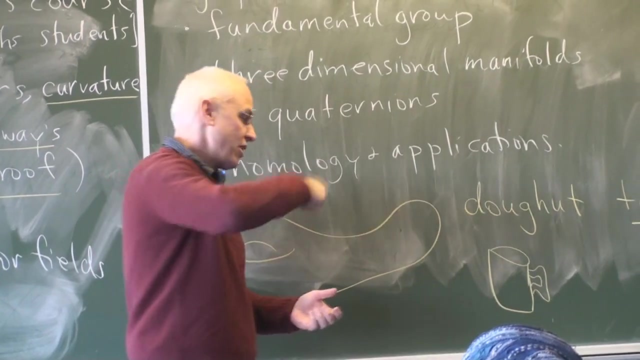 if you allow continuous deformation to a coffee mug, Can you see that This thing here is like the handle, And if I sort of punched my hole through the, If I punched my hand into the rest of it, I would get an indentation. 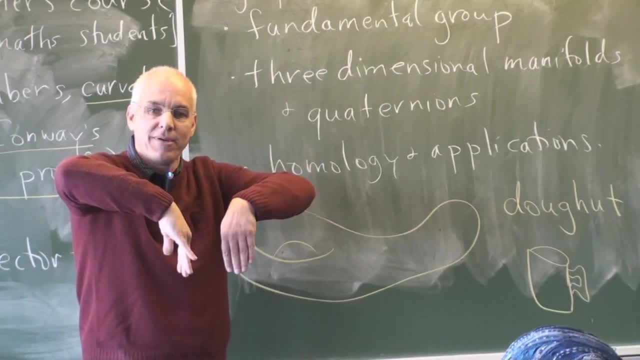 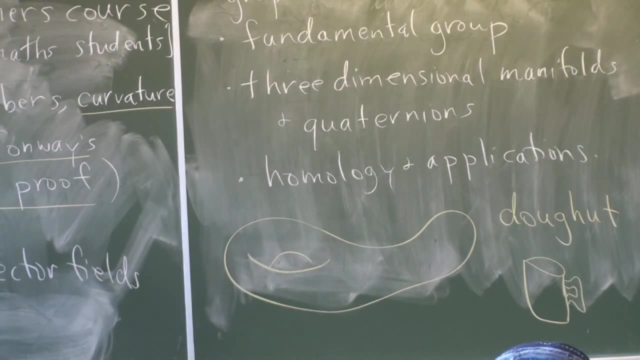 If I made that indentation sort of the shape of a cup and moved the handle around, then I would get a coffee cup. So the surface of a coffee cup or mug is, we say, homeomorphic? They are obviously not the same, Jimmy. 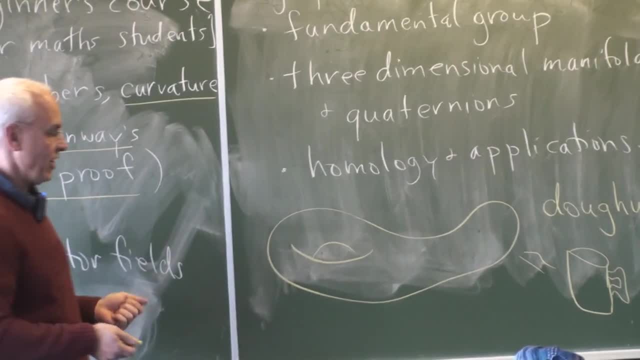 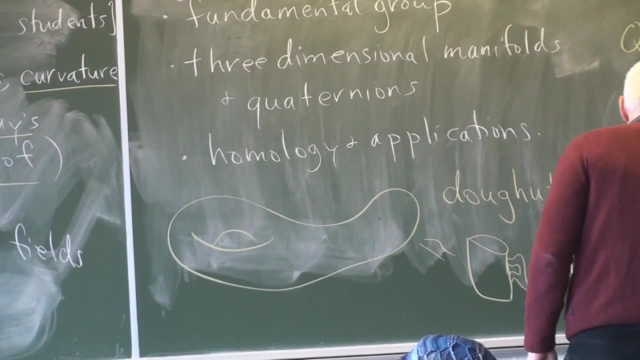 They are obviously not the same geometrically, but as far as topology is concerned they are the same. So these things are considered the same, and that's our notion of sameness. It's called homeomorphism. These are homeomorphic objects. 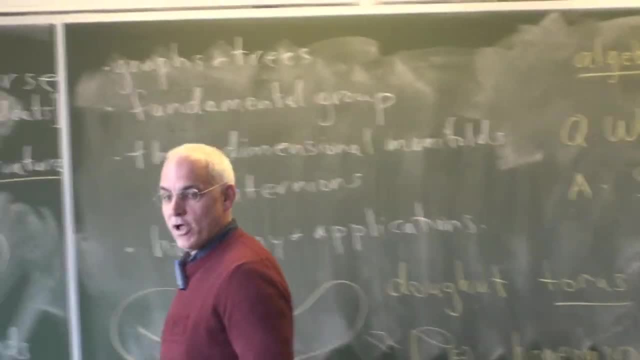 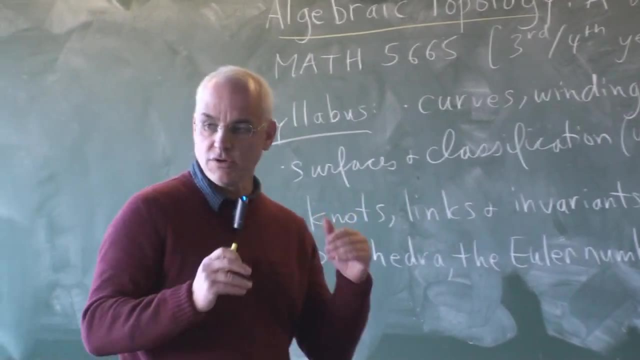 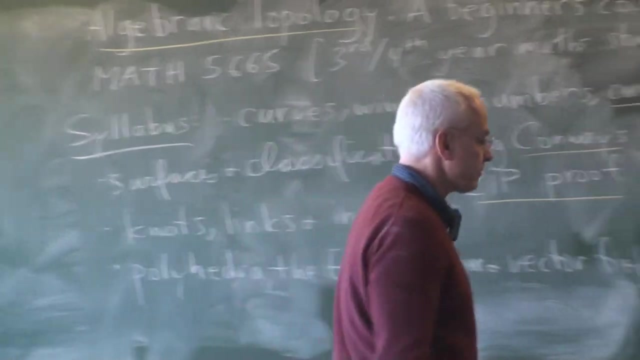 So this is not geometry. We are not interested in distance, We are not interested in making measurements exactly. We are interested in asking about what are the essential features of some mathematical objects which are invariant under this kind of continuous deformation. And one of the 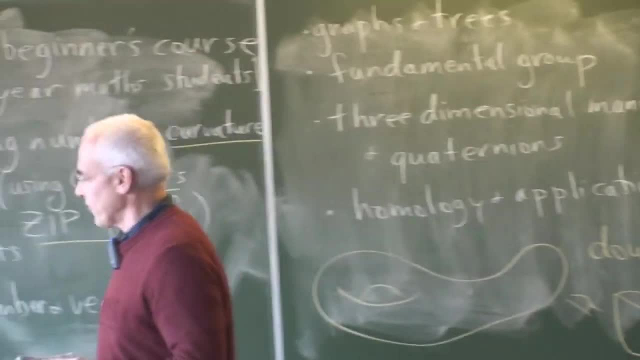 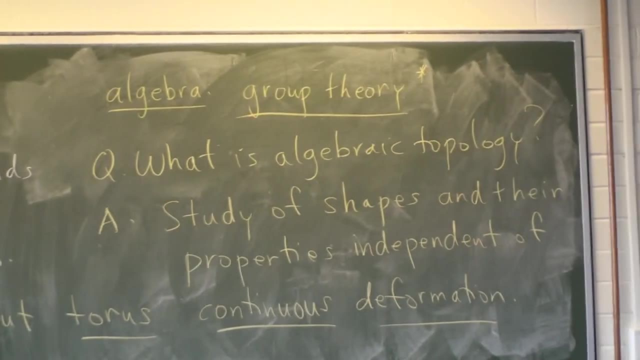 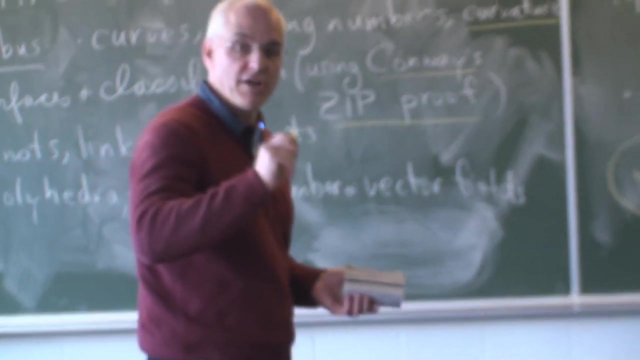 So one of the really important benefits of this course is that, yes, we're going to learn some algebraic topology and we're going to learn some particular techniques and concepts, But probably more important is that you're going to become familiar with a lot of really fundamental mathematical objects. 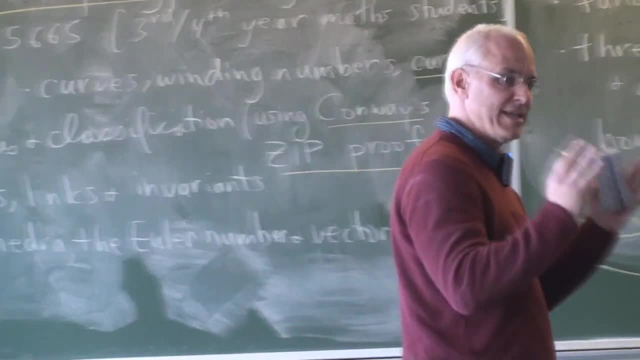 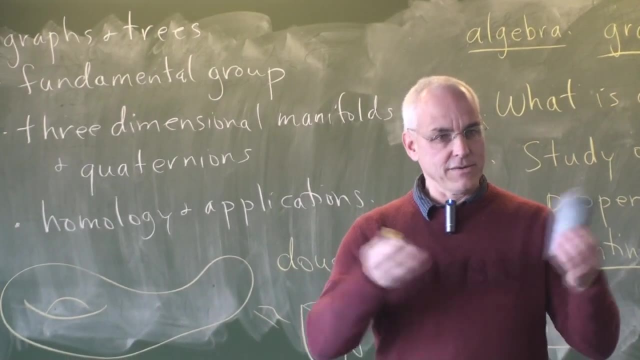 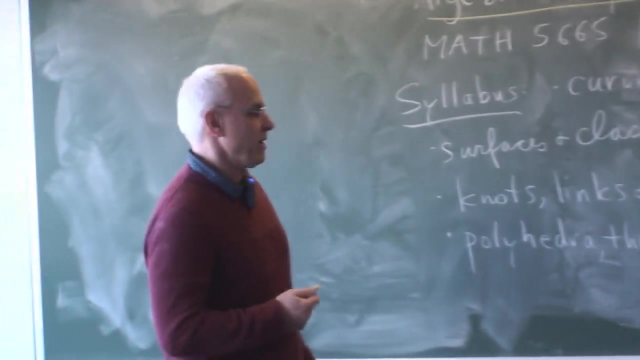 We're going to have a good look at some objects which are really central in mathematics, Because they're the ones that are the most interesting and they're the ones that people have looked at the most, And so that's probably almost for a student's perspective. 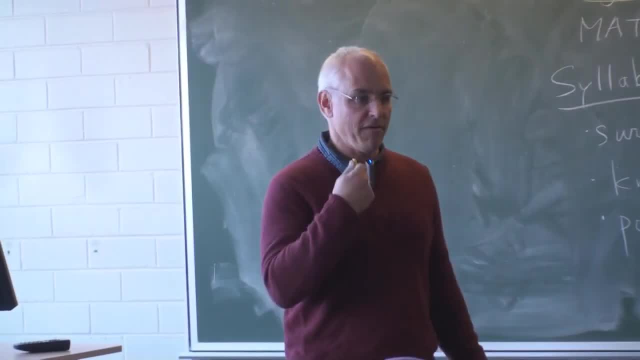 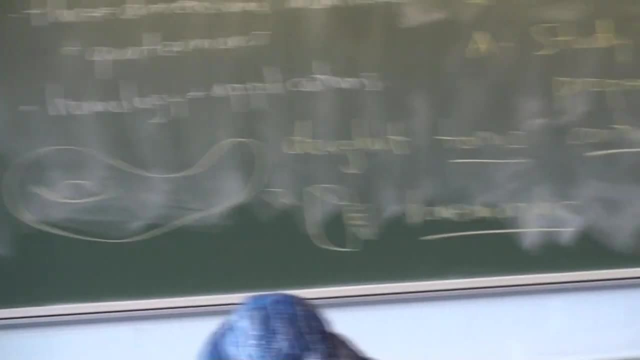 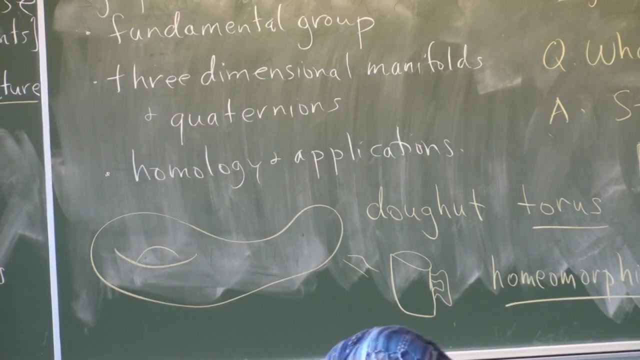 the most important thing that you might get out of this. You're going to learn about fundamental objects Such as what? Well, a torus is a kind of a fundamental object, As we'll see. It may seem rather arbitrary now, but you'll see that it's quite a fundamental object. 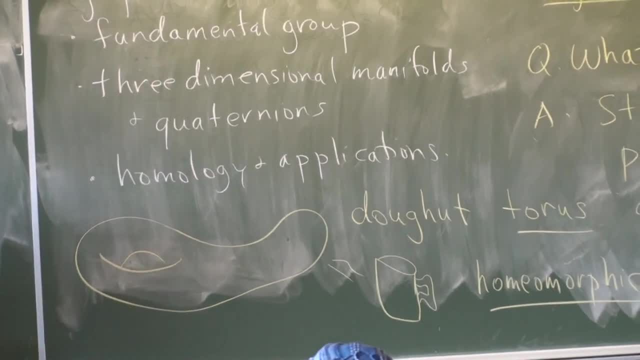 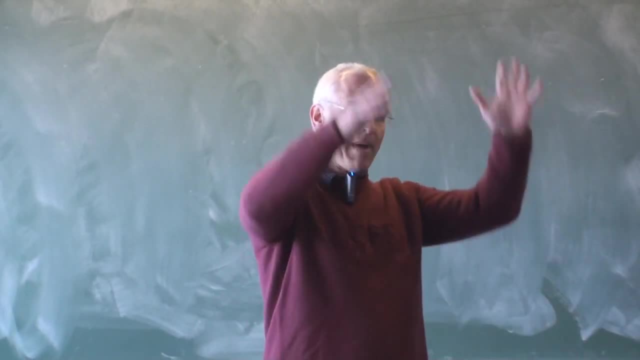 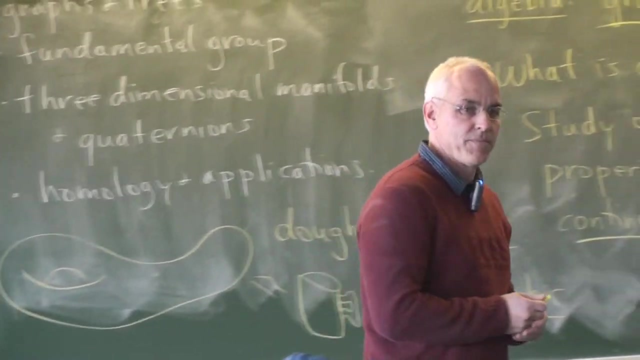 So let me ask you a question. If we had to choose what are the most fundamental mathematical objects of all the mathematical objects in the whole mathematical universe, what are the most fundamental mathematical objects? what would our answer be? Well, there's lots of. 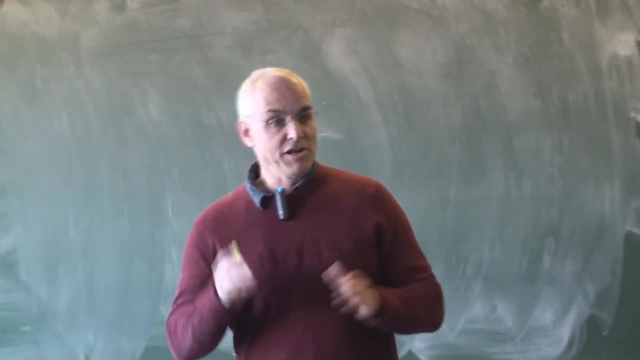 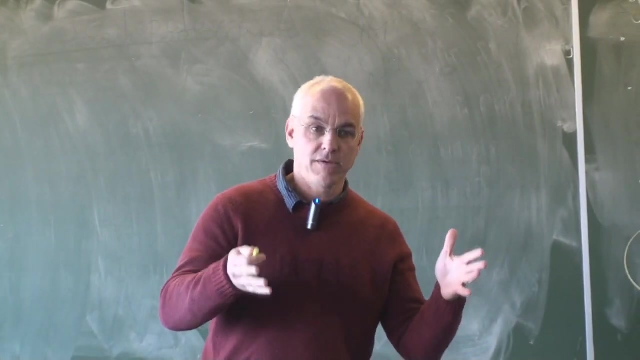 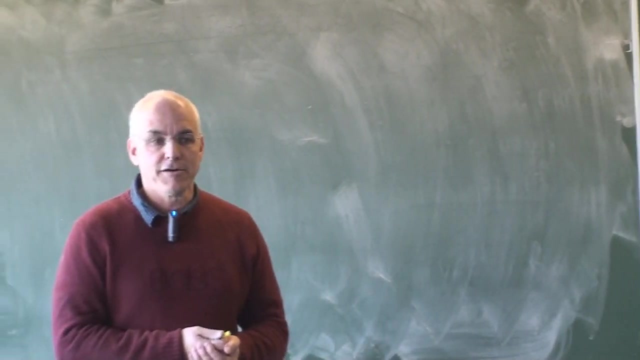 different possibilities. Maybe it sort of depends on what you consider important or what you consider fundamental, But certainly we would want something that's historically important, that's been studied for a long time, Something that has a very rich theory, And so what would your guess be? 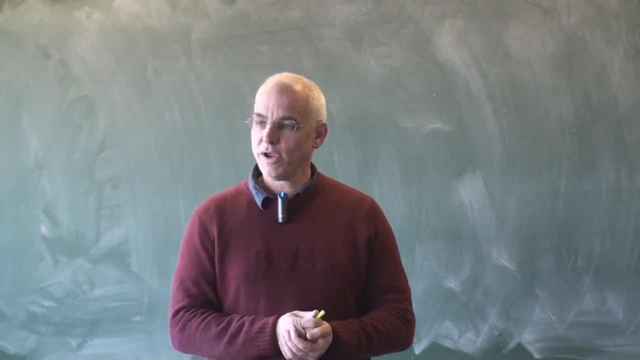 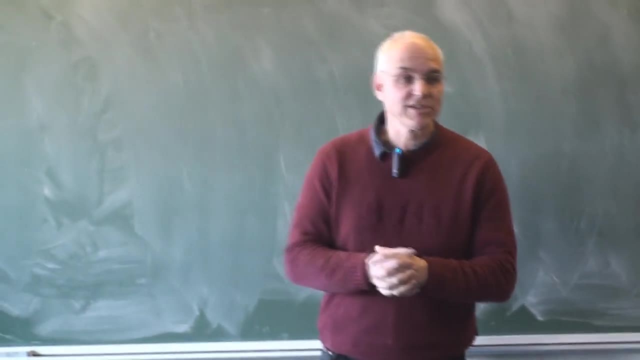 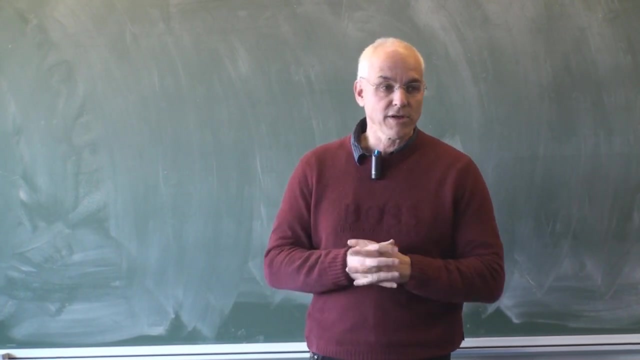 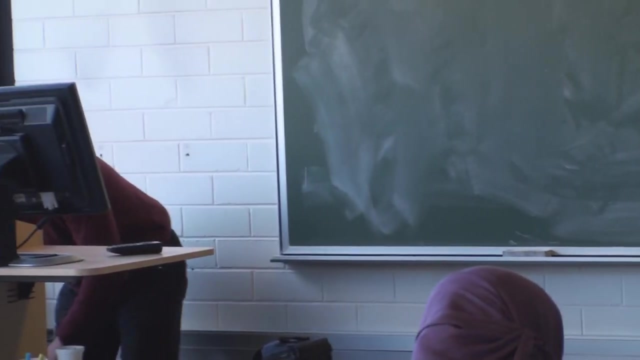 A sphere. Anybody agree? I think a sphere would be certainly a candidate. I've in fact brought what I think are the two most important historically and interest-wise, the two most important mathematical objects. I brought them along today, And one of them is a sphere. 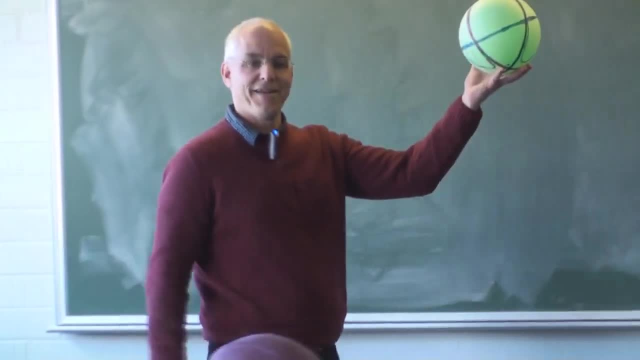 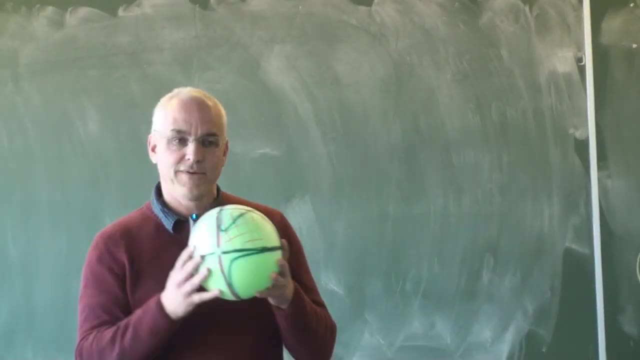 It's maybe not such an impressive sphere, but okay. So that's a sphere And you're all familiar with the sphere And you're all familiar with at least some of its geometrical properties. But of course that's also a sphere now in topology. 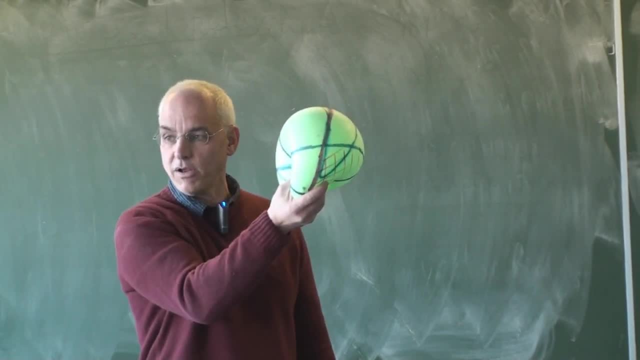 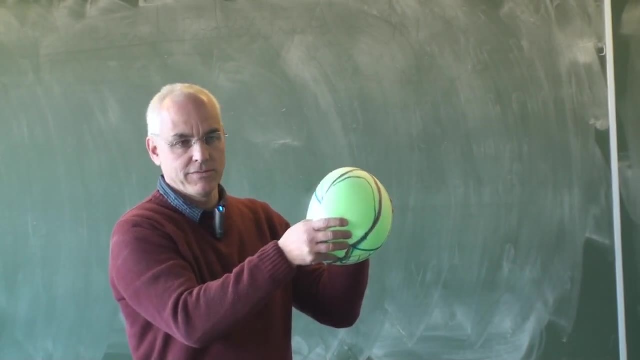 It's not a sphere in geometry, but that's also a sphere in topology. So all those beautiful properties of the sphere that depend on the geometry are not going to be that much of interest to us, But nevertheless that's certainly one of the most important. 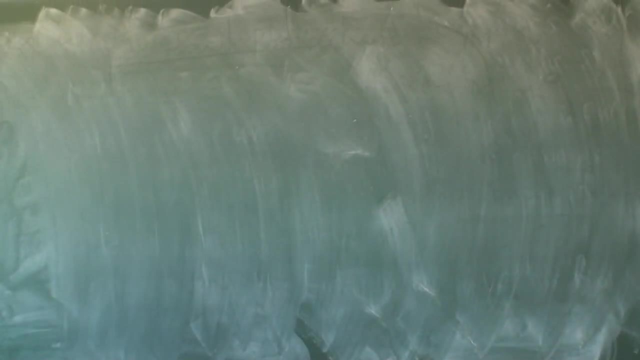 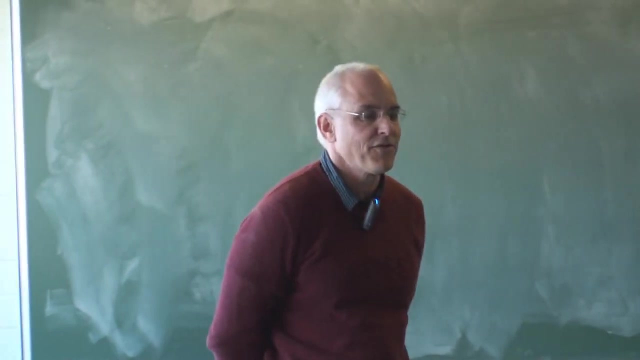 mathematical objects, And I've got a second one in here. What's the other one? No, Not so interesting. Yes, it's important, of course, but it doesn't get the heart racing like a sphere. You know, a sphere is kind of exciting. 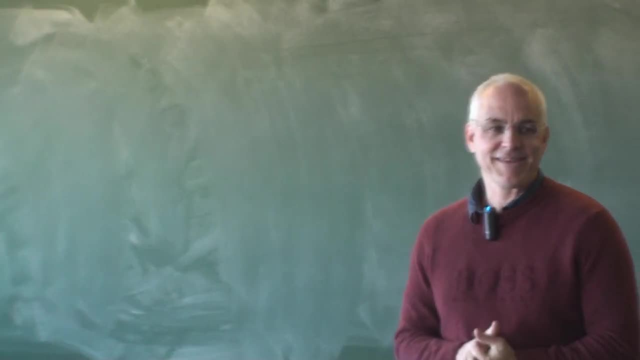 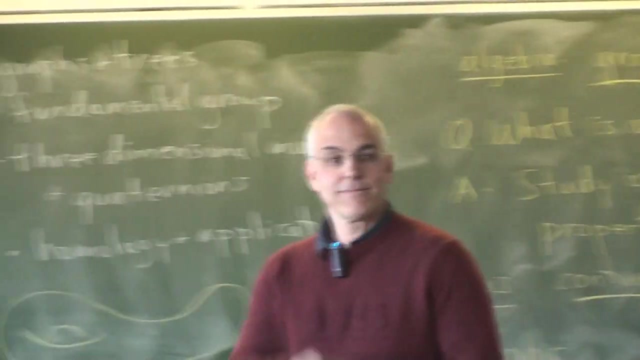 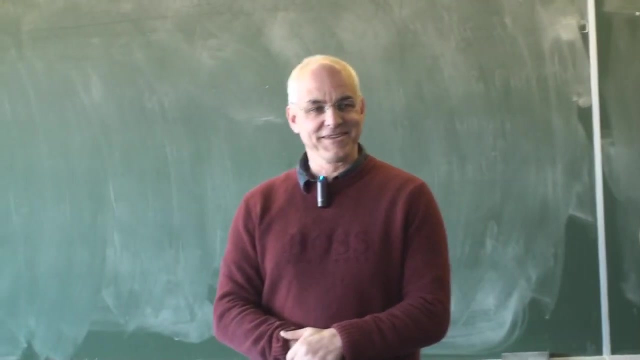 A parabola. A parabola is a good choice, but something more, I think, ultimately more historically interesting. Yes, A torus, A torus, That's also a good choice, But I think what I've got in the bag beats a torus. 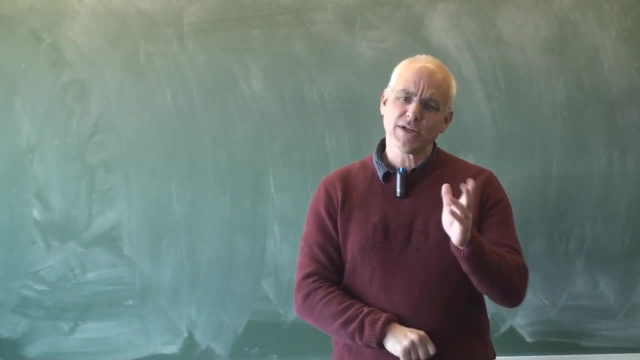 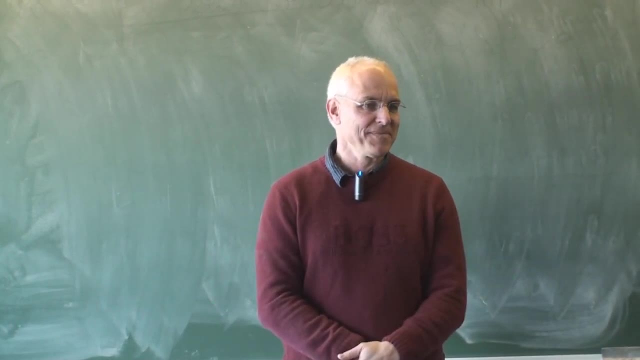 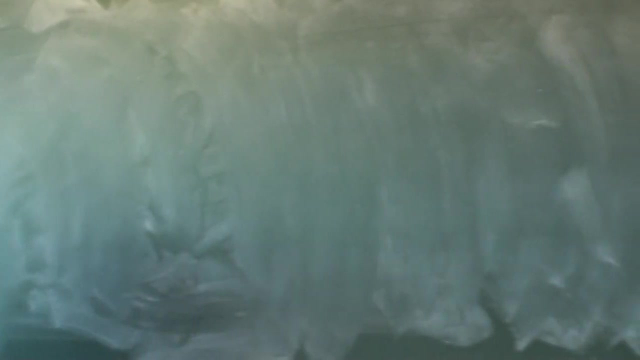 A mobius band. A mobius band- another good choice. but it was only developed in the late 19th century or middle 19th century, so it historically doesn't have such a right for this high elevation Drum roll. and I'll show it to you. 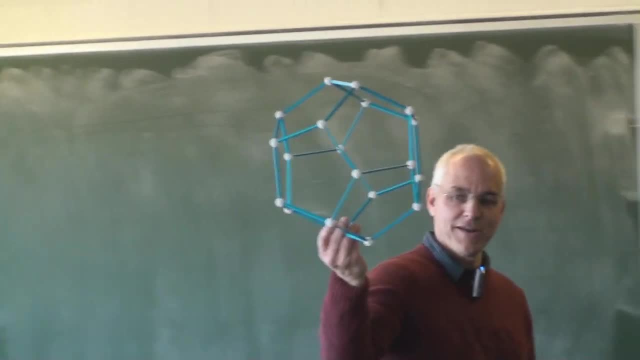 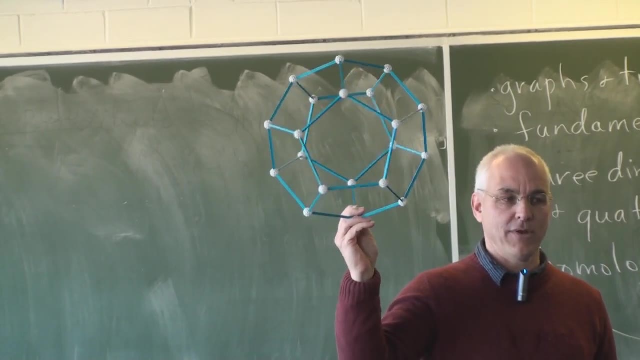 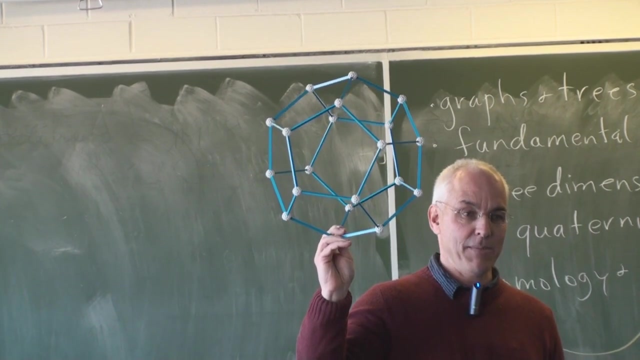 Yeah, it was right there. Do you know what it is? It's a dodecahedron. A dodecahedron. Isn't that the same as a sphere? Topologically it is. It is the same as a sphere. 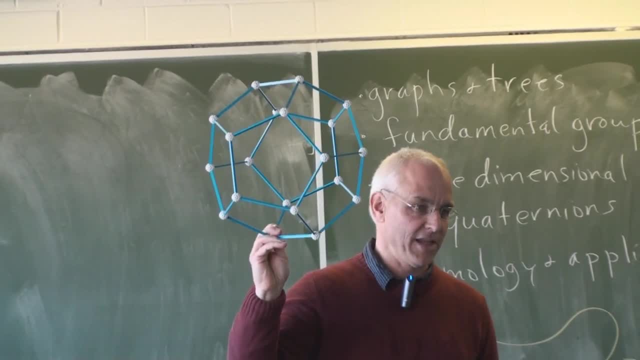 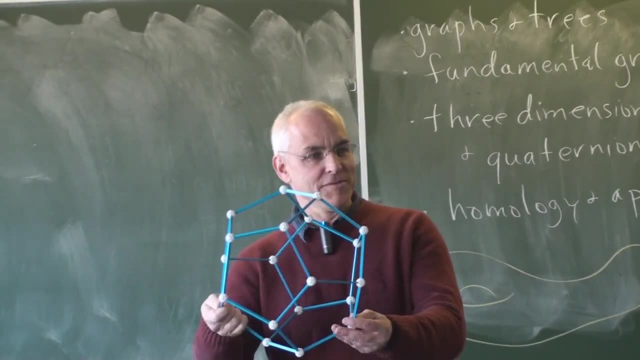 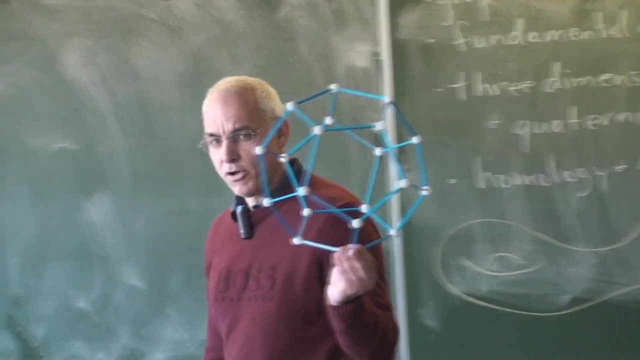 But that's only an idea that's about 100 or 150 years old, And only if you're in an algebraic topology class. If you're in a combinatorics class or a differential geometry class, it's quite different. Now I hope you all know that this is one of the five platonic solids. 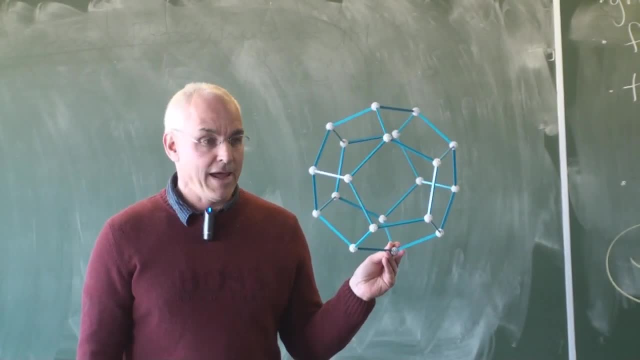 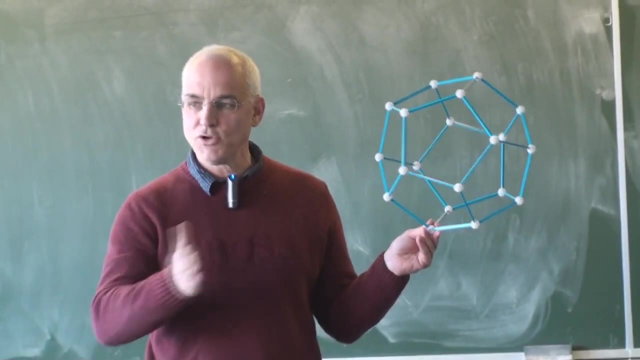 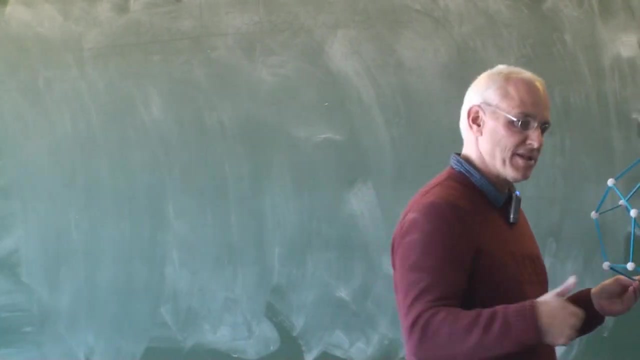 There are actually five of these things And they were of paramount interest to the ancient Greeks. Euclid, I remind you, wrote the book The Elements And it's got 13 volumes And it's presentation of all of geometry that the ancient Greeks knew. 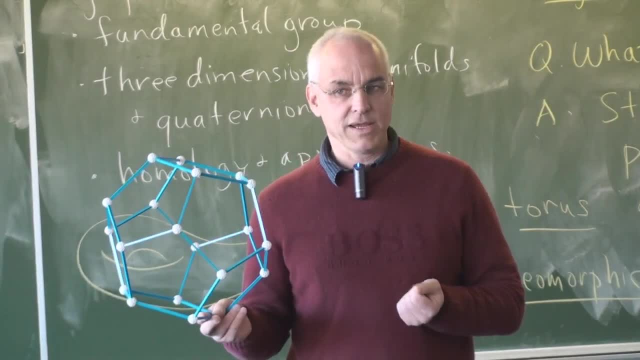 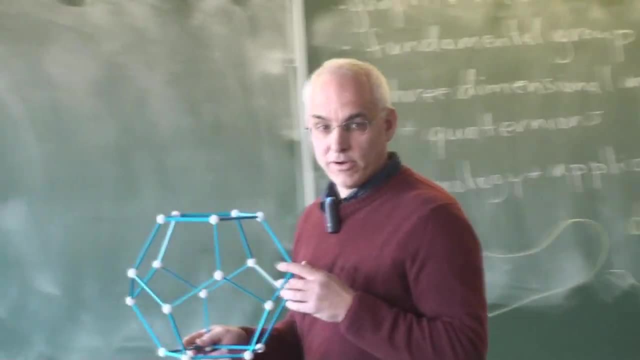 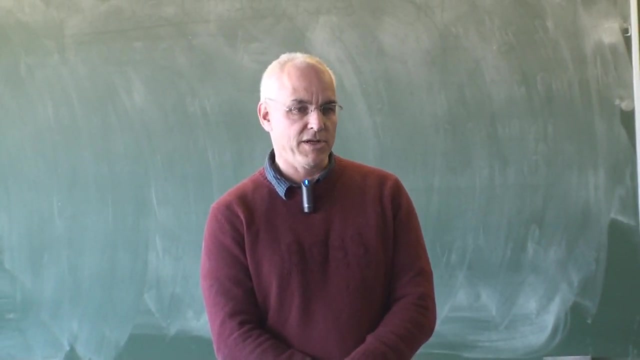 And the culmination of Euclid's work is in the 13th book is a study of the platonic solids. It's the high point as far as Euclid was concerned, And this particular one is historically the most important of all: the platonic solids. 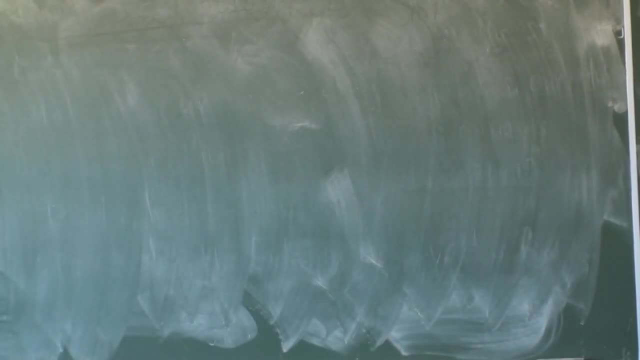 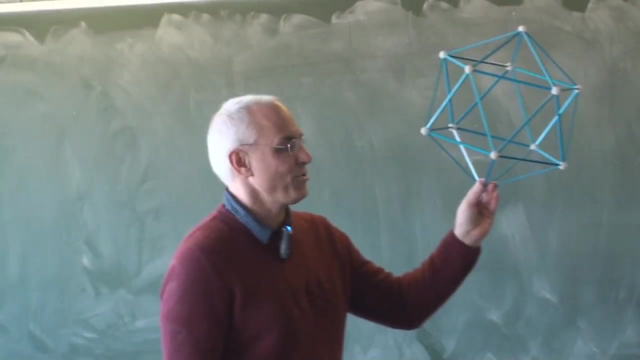 I don't have all of them with me today, But I do have another one which is also quite interesting. What's this? one called The icosahedron? Icosa, I think, refers to 20.. This has 20 faces. 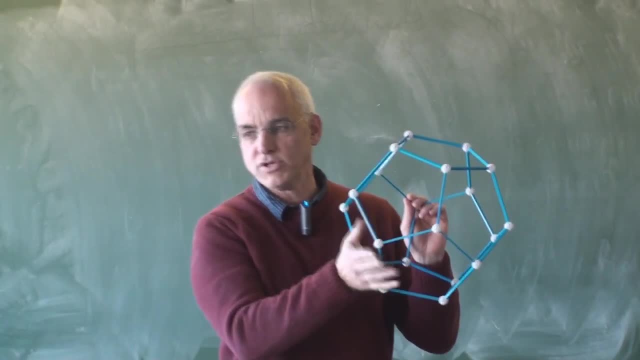 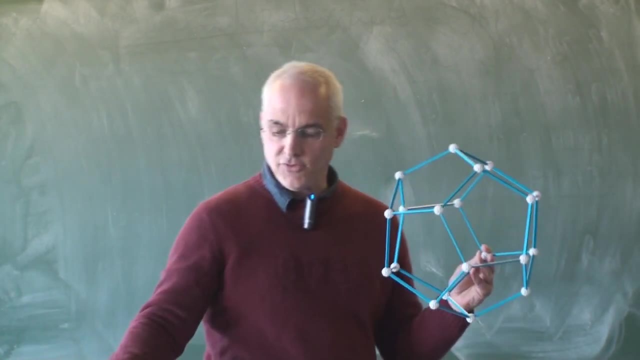 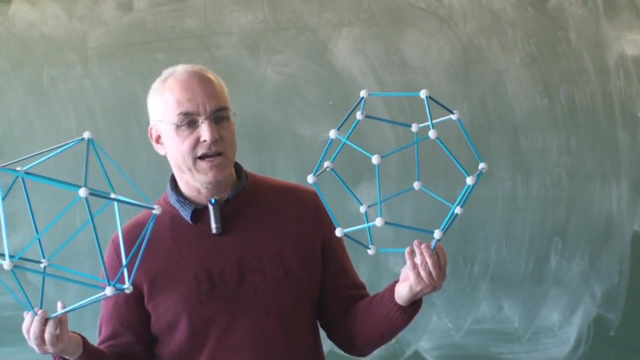 They're all triangles. Dodeca comes from the Greek. Dodeca means 12. It's got 12 faces. This one's got 20 vertices. This one's got 12 vertices. These are dual in a very precise sense. 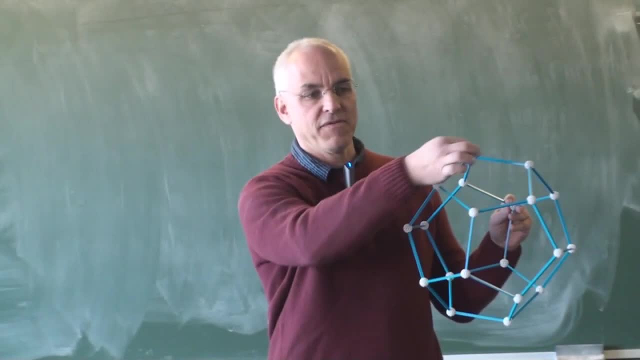 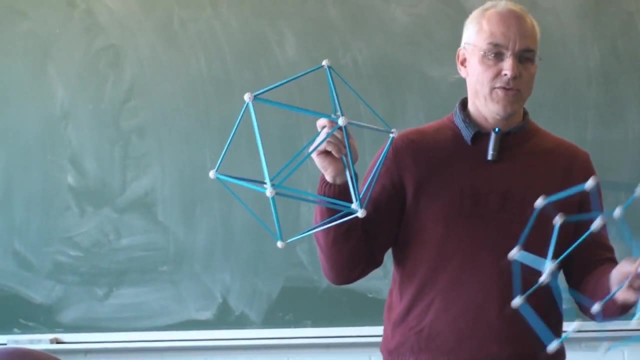 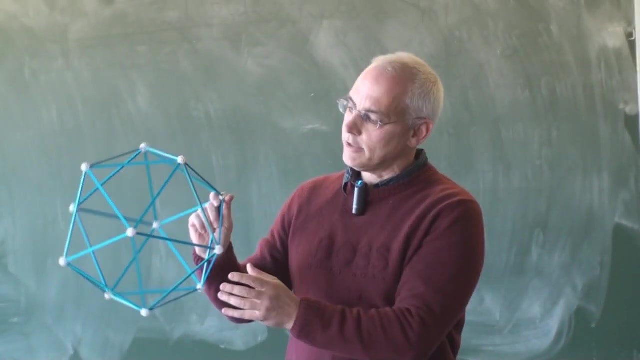 In the sense that if you take the centers of the faces here, well, you get 12 vertices which are forming an icosahedron, And conversely, if you take the centers of the faces here, then you get 20 points which form a dodecahedron. 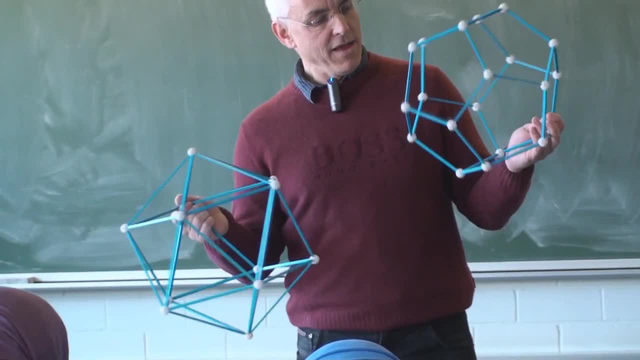 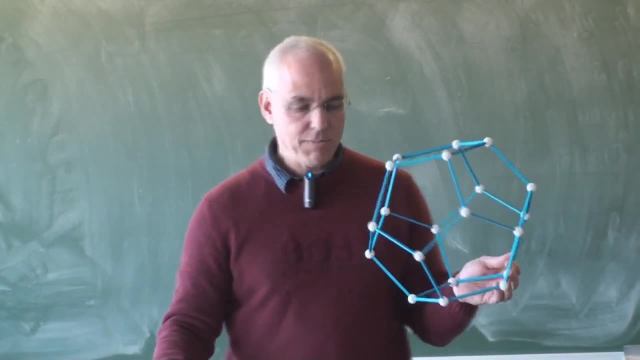 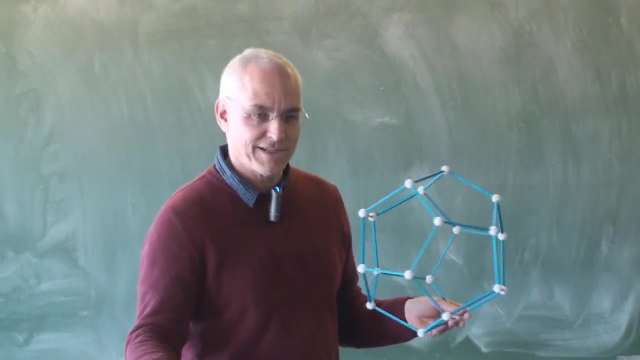 So they're dual. So why then, have people historically considered the dodecahedron to be somewhat most important? It's because this one is a little bit rounder. If you had to play soccer with one of these two things, you would be best off choosing this one. 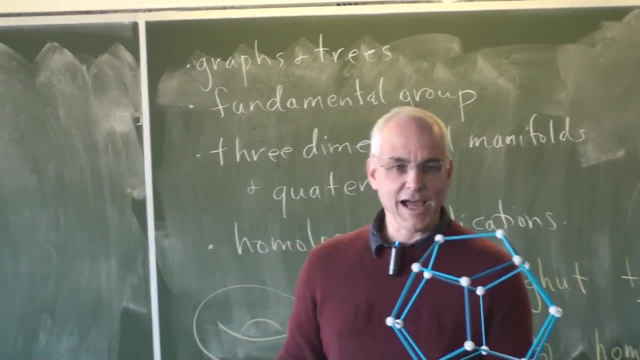 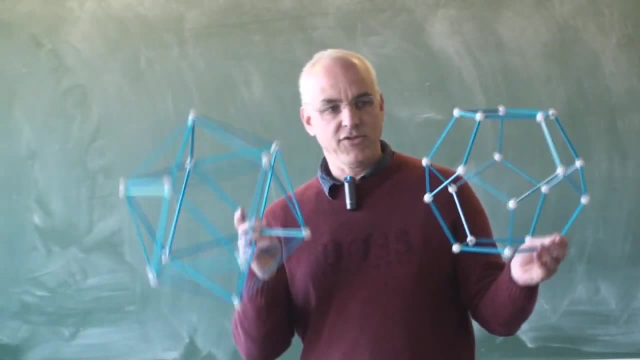 You can try it- Not with these, because they wouldn't last very long under rigorous FIFA conditions. But if there was actually a ball made like this, you would much prefer to play with this one. It's rounder And we're going to talk about that when we talk about curvature. 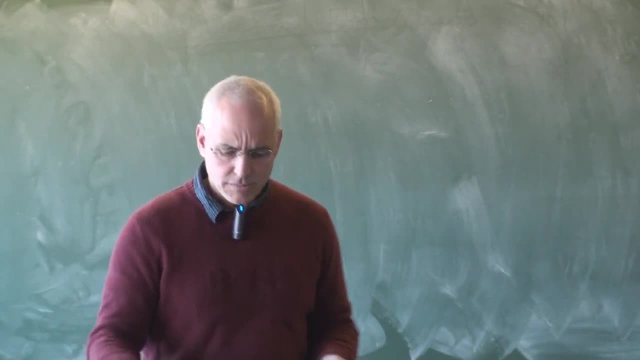 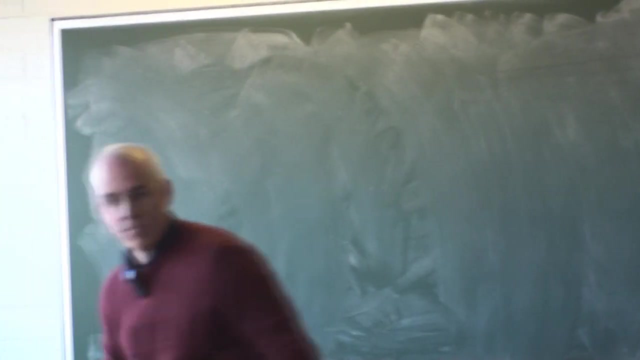 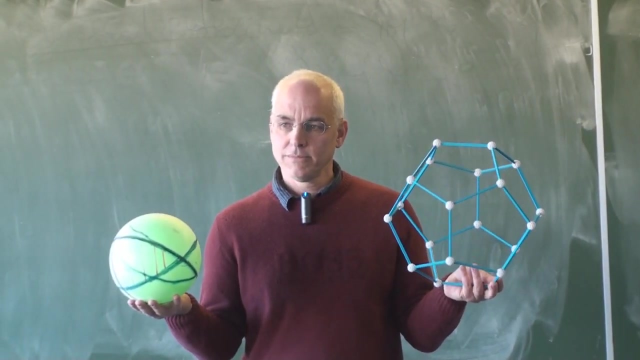 How does one assess roundness? But in algebraic topology, let's put this one away as a secondary object. So here are my candidates for the two most important historical objects, And I think it's hard to choose between them. They're both really interesting. 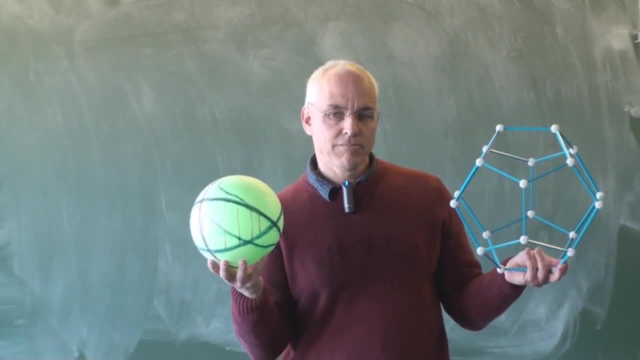 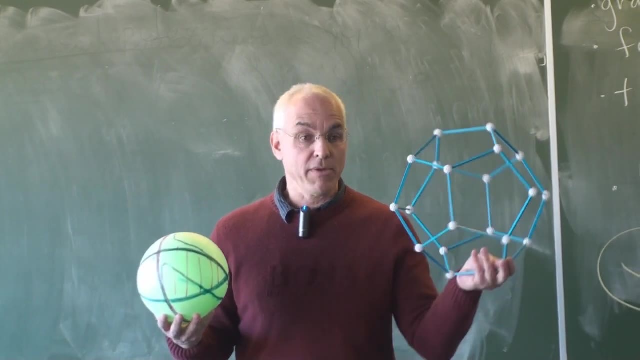 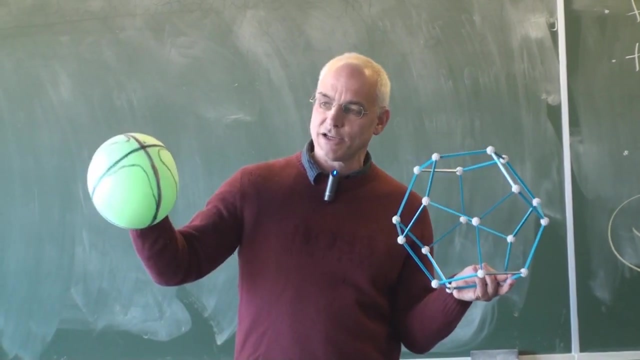 If you're an analyst or a geometer, perhaps this is more important or interesting. If you're an algebraically minded person or combinatorially minded, you much prefer this one, And in some sense this is a continuous approximation of that one. 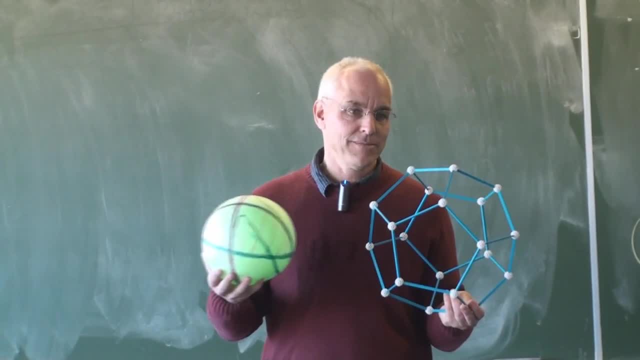 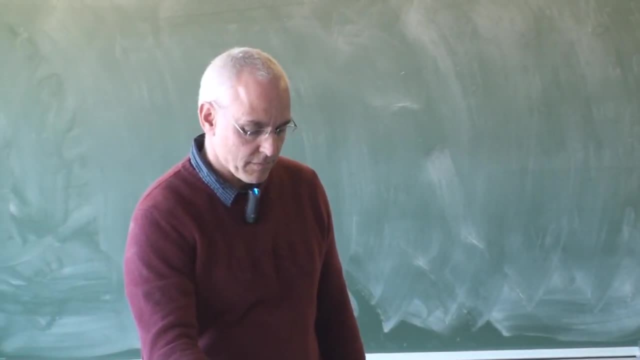 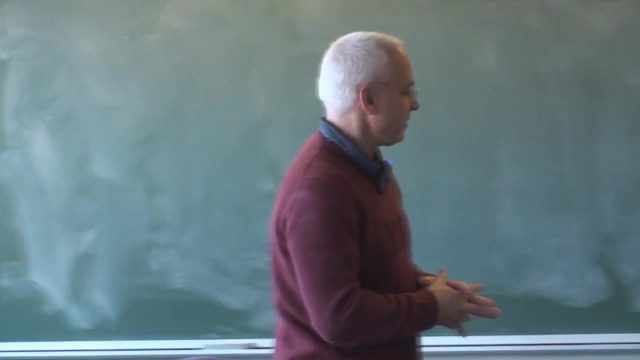 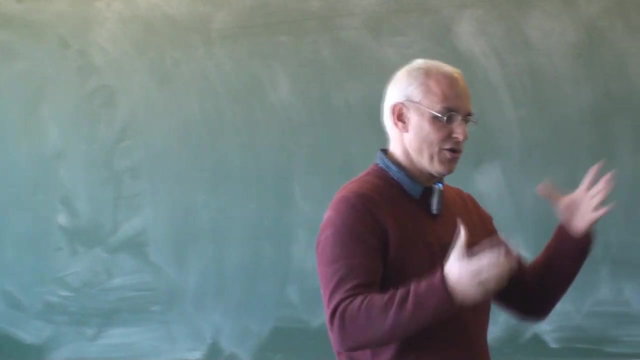 And this is a discrete approximation of this one, And the interplay between these two things is something that's going to be important to us. Alright, so there's lots of other interesting things that we're going to be talking about, And topologists like to argue physically. 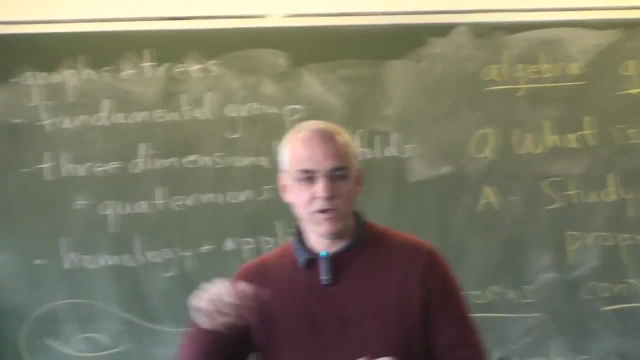 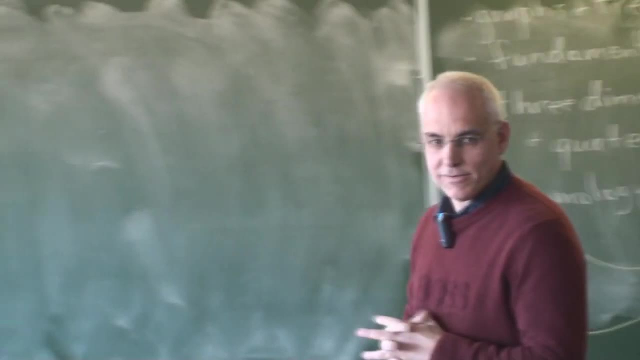 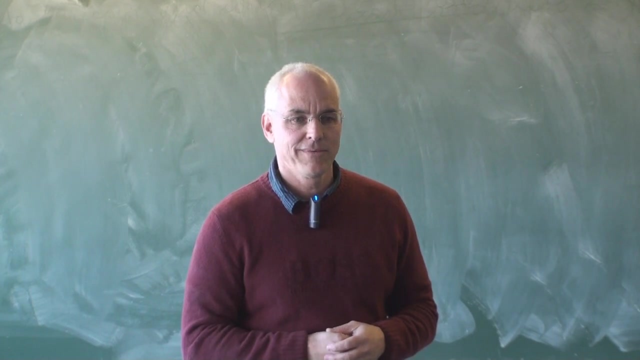 Topology is a subject which is often a little bit dubious. logically, I have to say that to be quite honest, because many of you know that I'm a bit fussy about mathematical foundations, And there will be many times in this course where we have to argue by pictures. 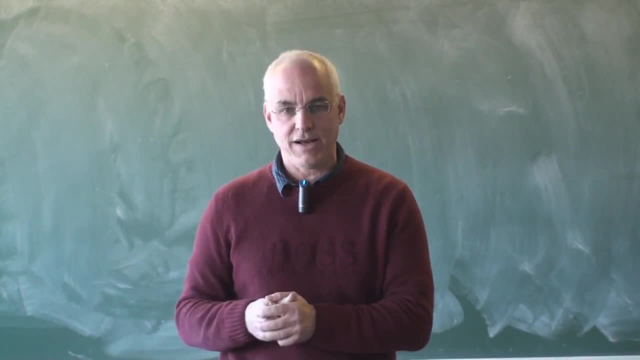 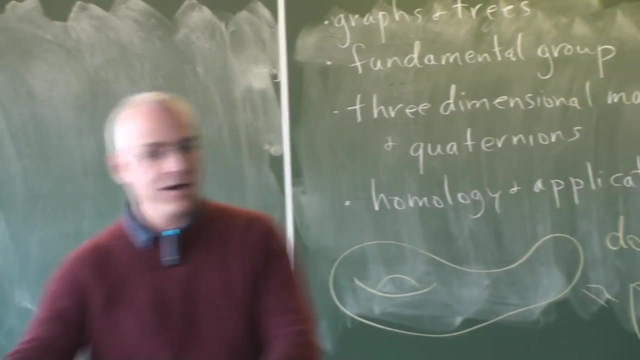 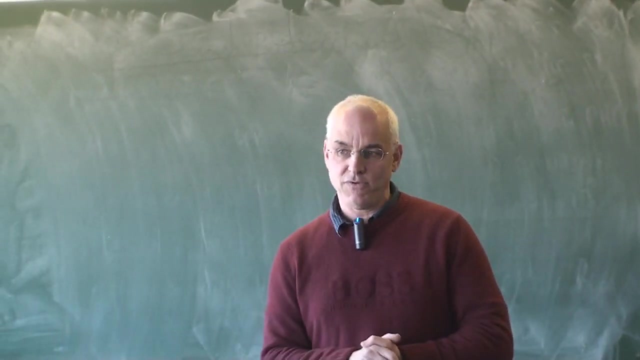 The nature of the subject is different from any other subject you've done in mathematics. We'll argue with pictures. we'll argue with intuition, by analogy, by making a model and saying: look, Okay, So we're going to have sort of an engineering or applied mathematics point of view on things. 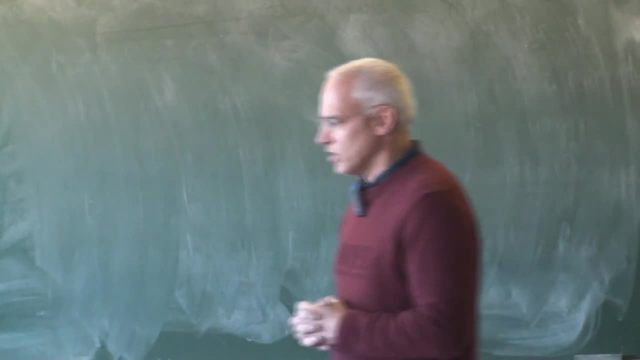 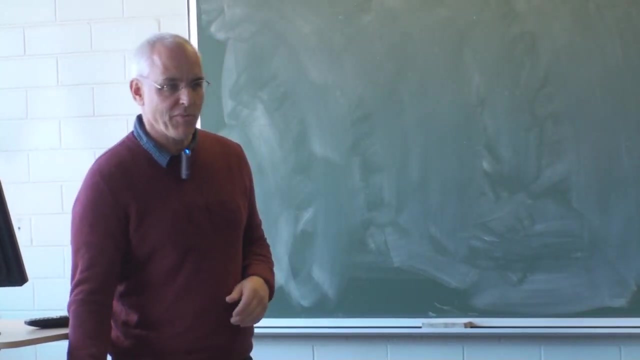 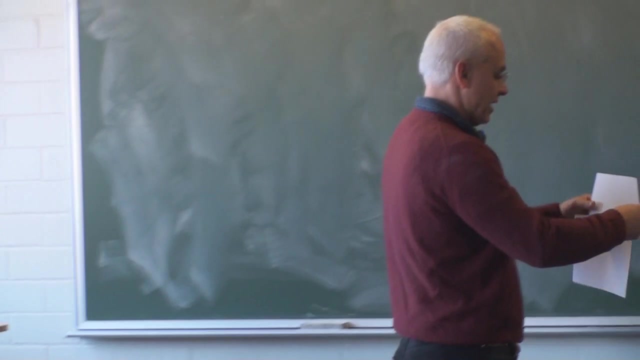 And when it comes to actually laying the foundations, that's a little bit challenging sometimes. So I'm going to give you some problems to think about. These are all sort of standard problems, but they're good to get started. So problem number one concerns this object right here. 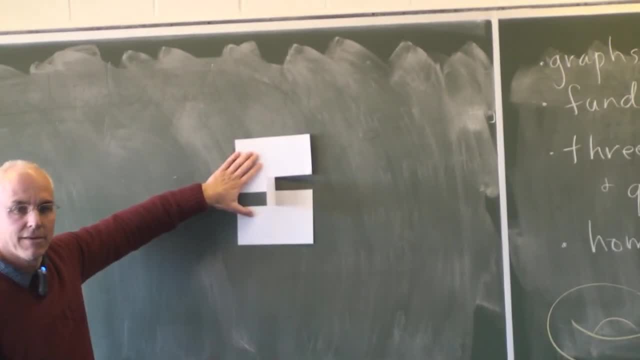 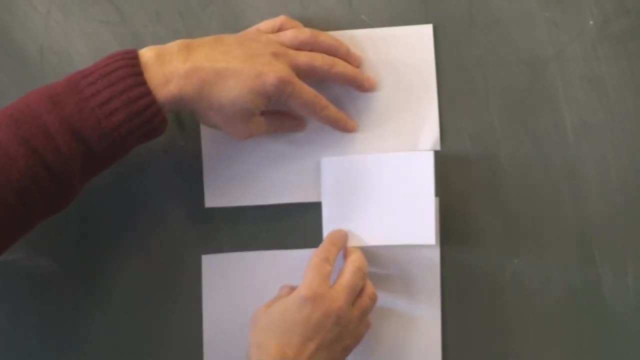 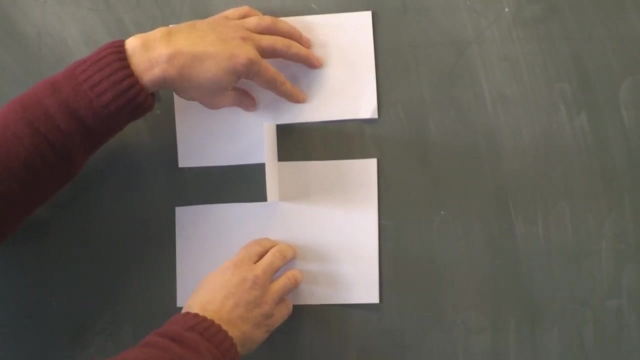 Okay, Can you see that? Does it look interesting? Okay, it's got a flap. Okay, It just flaps there. There's nothing hidden about it, And I made it out of a single piece of paper, Without any glue or 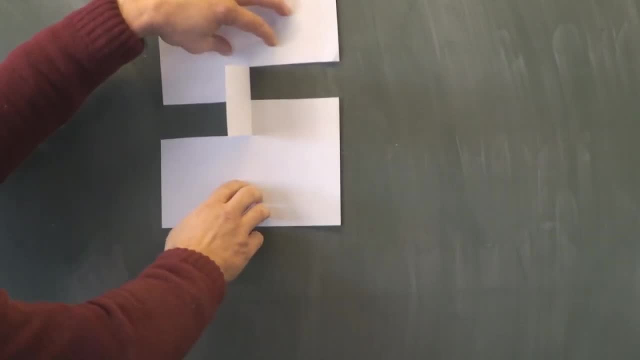 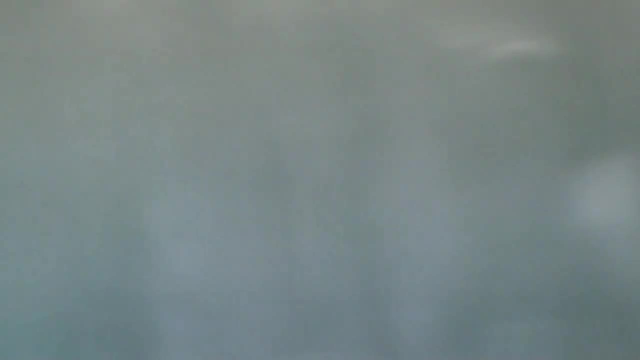 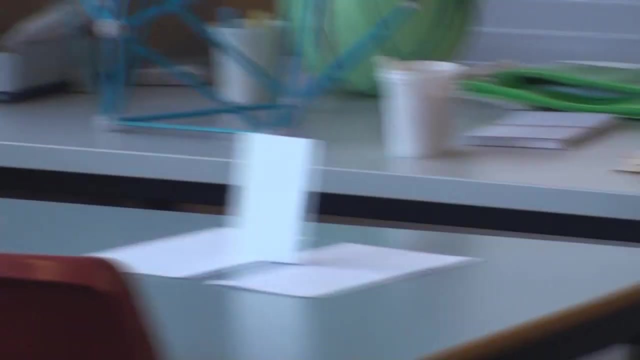 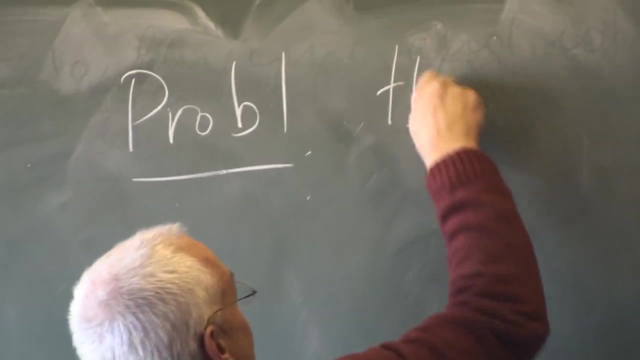 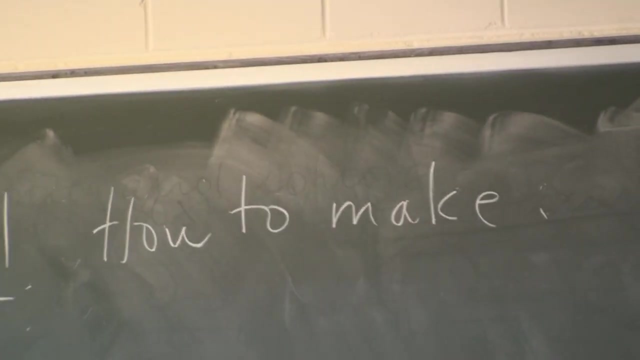 I just made some cuts and made this. So the first problem is: how do you make such a thing? Okay, So maybe I'll put it over here. Okay so that's problem number one. Problem one: How to make. Okay, now I have to draw this thing. 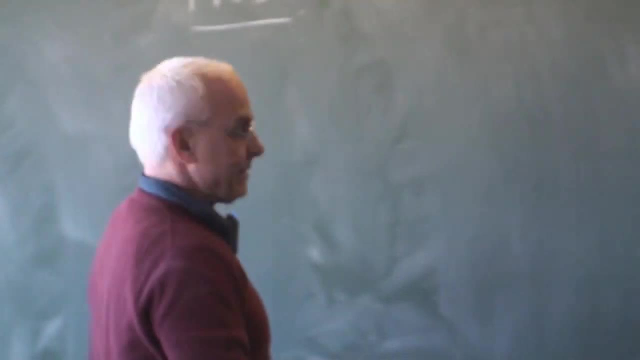 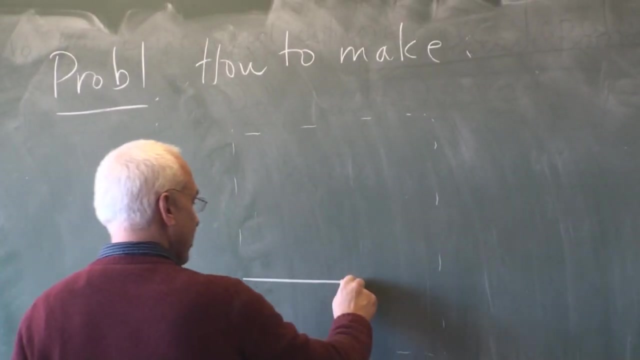 Well, I've already done it, so the video camera's already got it, but I have to draw it anyway, Okay. so this might be a little bit challenging. So there's, roughly It's got something like that, Okay. So there's sort of a piece that goes up like this: 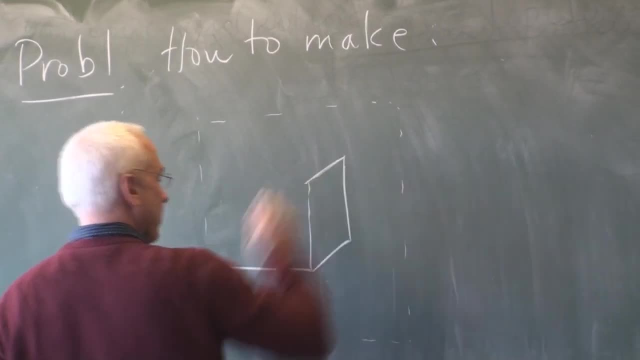 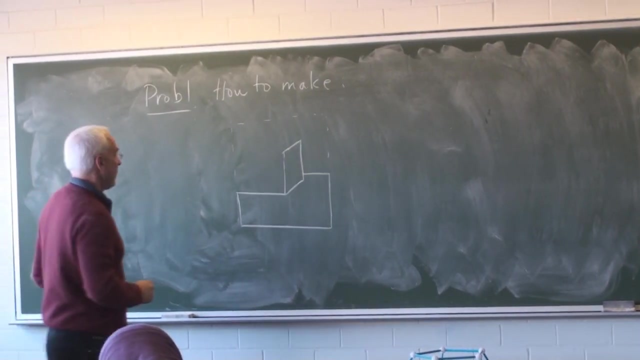 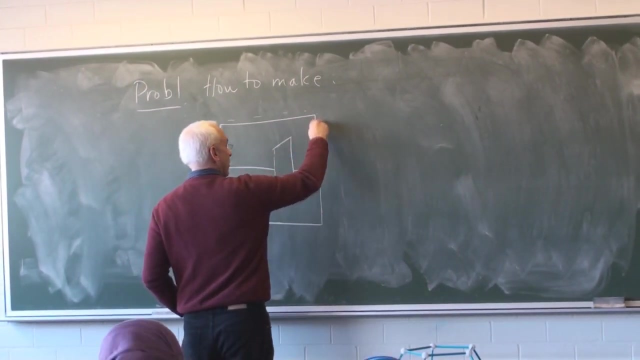 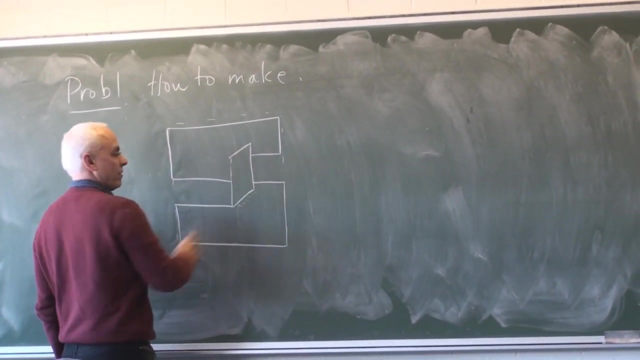 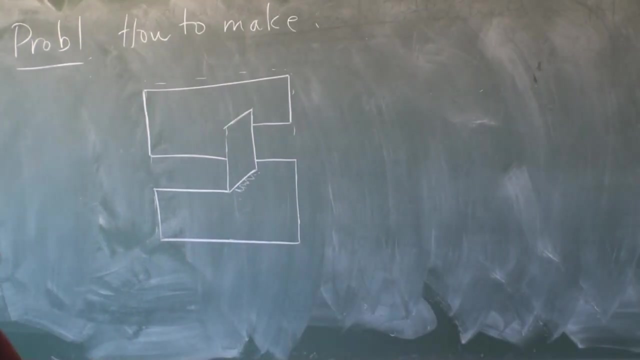 and then there's this fold- Maybe the fold will be like that. And then there's a piece that goes like this, And then the other piece all carries on like this: Okay, So this is the fold here. Does that look like it? 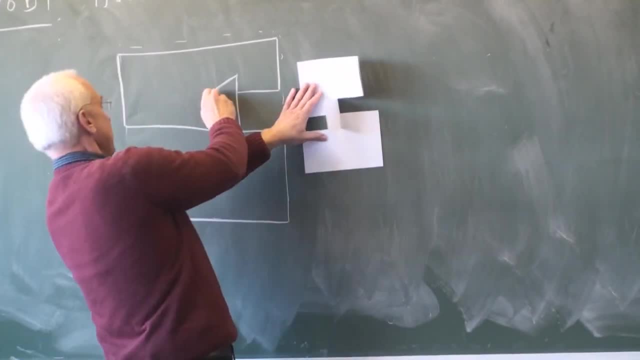 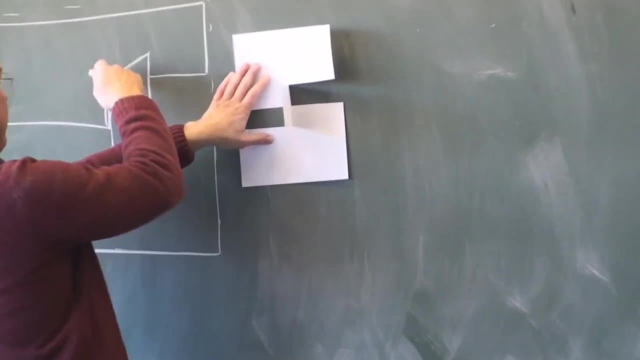 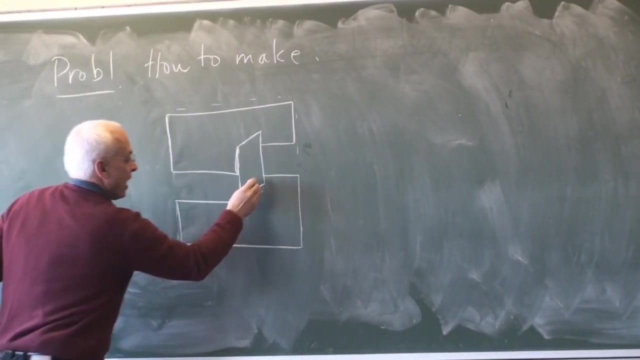 Can you explain the fold? Yeah, okay, So there's a fold here and there's kind of a fold on this side, So that part comes up to that fold and that part comes up to that fold. So, okay, behind here there's something. 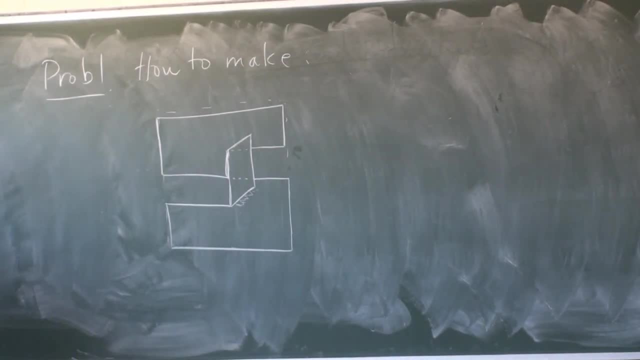 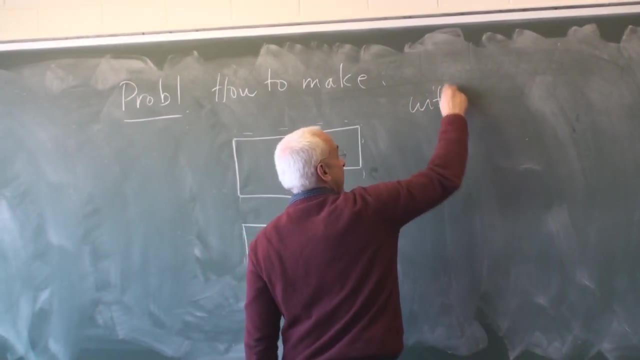 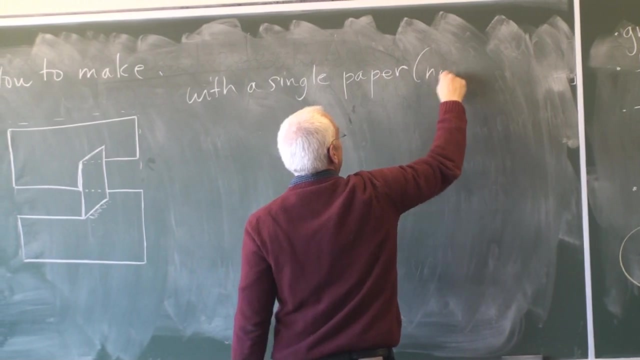 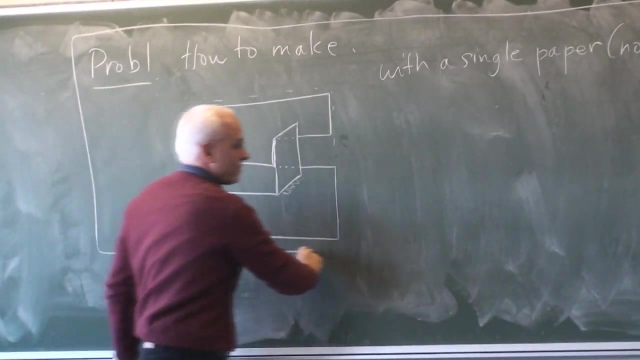 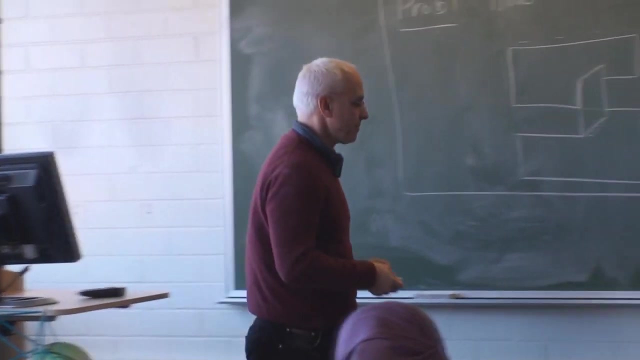 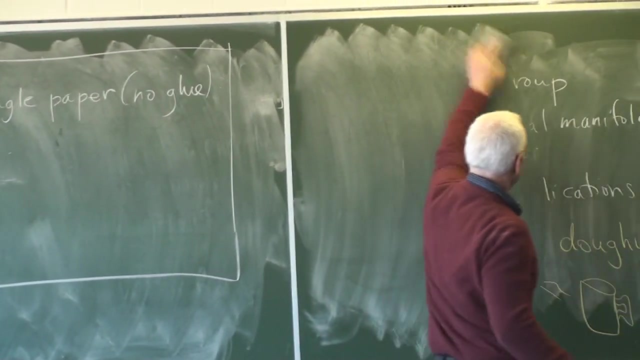 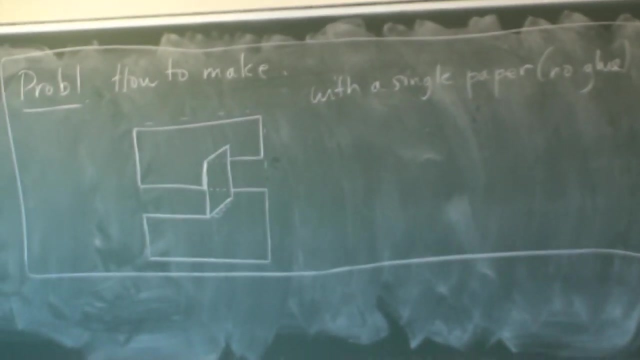 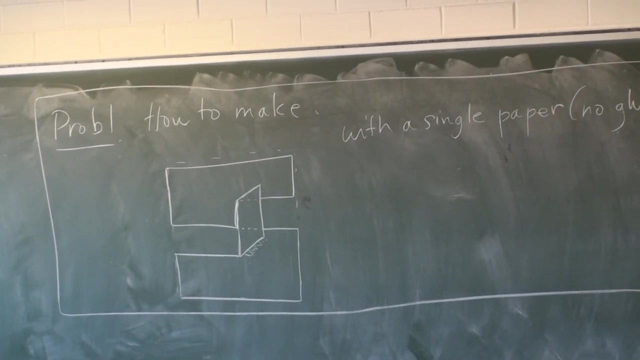 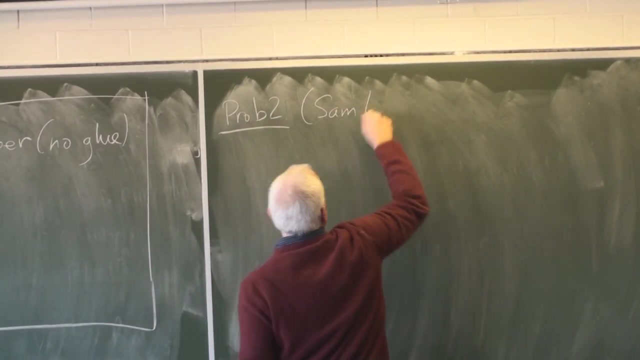 Okay, How to make this with a single paper And no glue. So there's problem number one, Okay, And here's problem number two. And here's problem number two, Okay. this goes back to a famous 19th century puzzle maker. 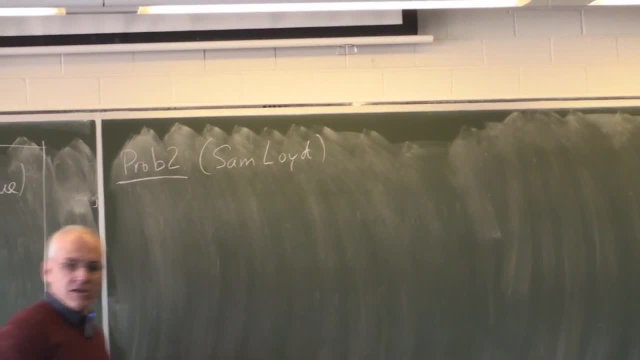 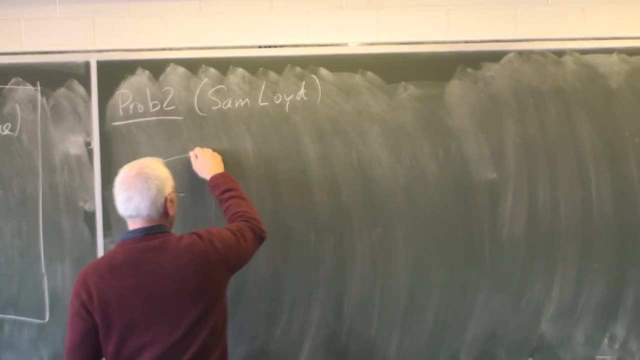 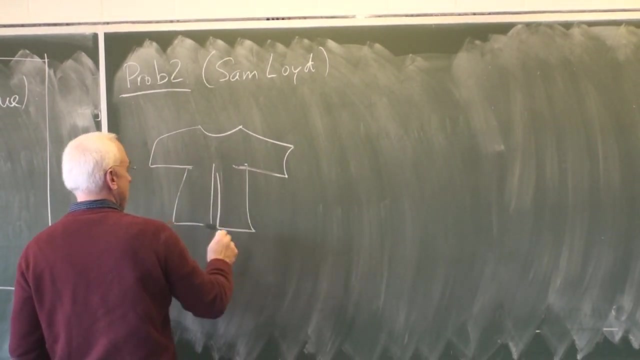 named Sam Lloyd, who also created lots of chess puzzles and other things. So what you do is you have The ingredients. are you need a shirt with lots of buttons and holes for the buttons? with lots of buttons and holes for the buttons? 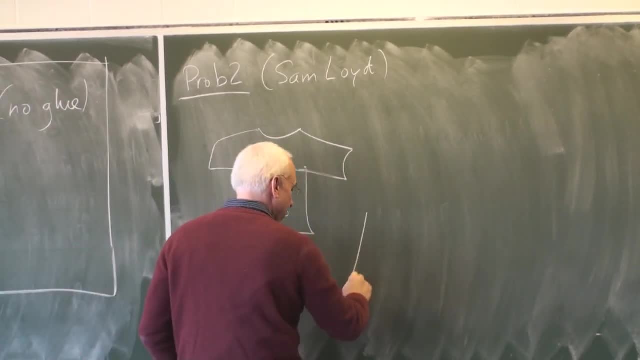 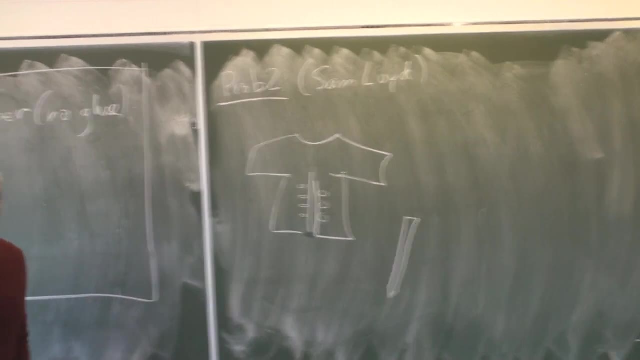 Okay, And you also need a pencil. Well, it doesn't have to be that big, but okay, It's in large view. There's a pencil And from the pencil you have a loop. You've got a piece of string. 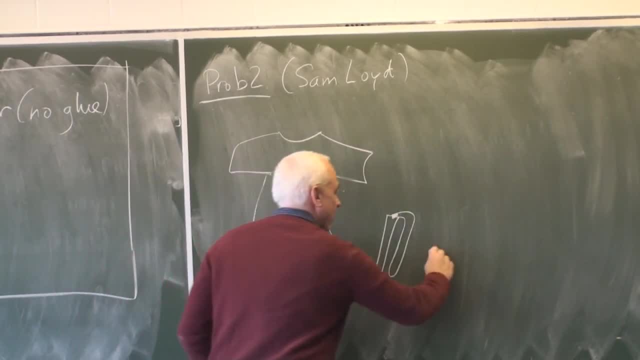 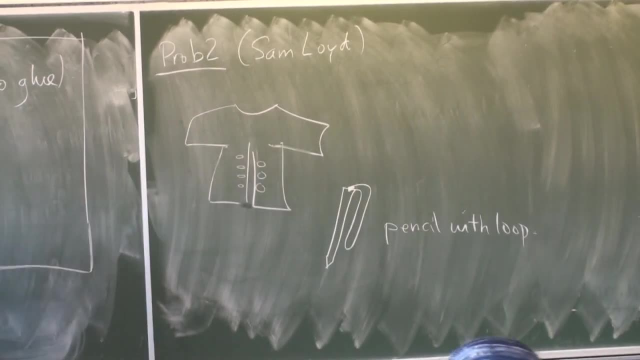 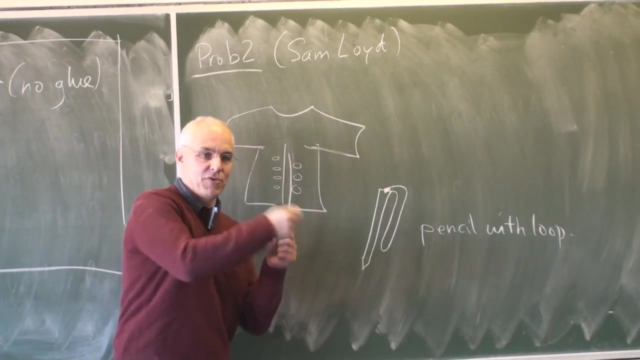 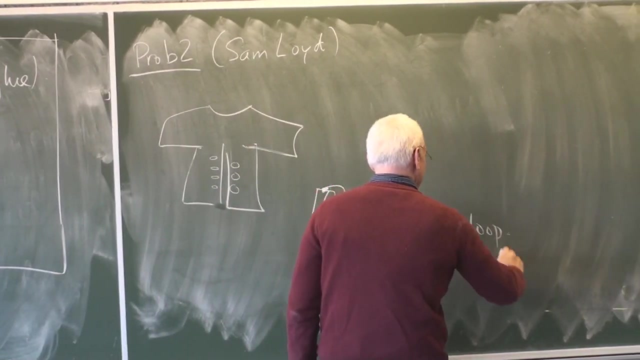 which is looped like this. So this is a pencil with a loop And the loop is not big enough to go over the pencil. Okay, even if you pull it tight, it's not big enough to go over the pencil. So, with a loop which is smaller than the pencil, 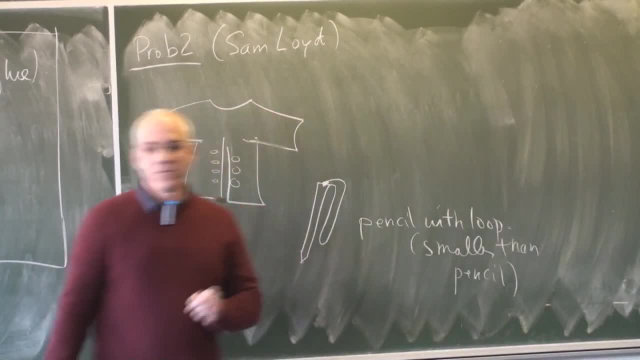 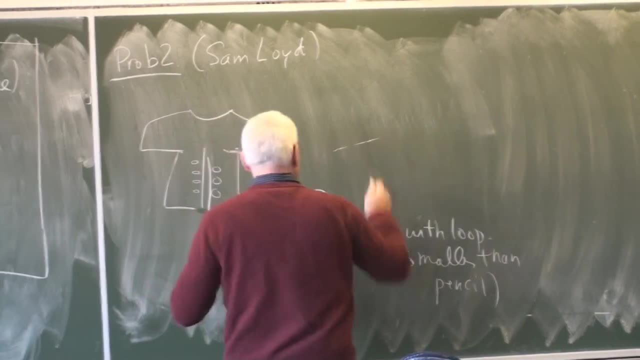 Okay, And so these are the ingredients, And then what we do is, if you know how to do it, what you do is you take the shirt and you can actually do it on with somebody's shirt If you have one of these things. 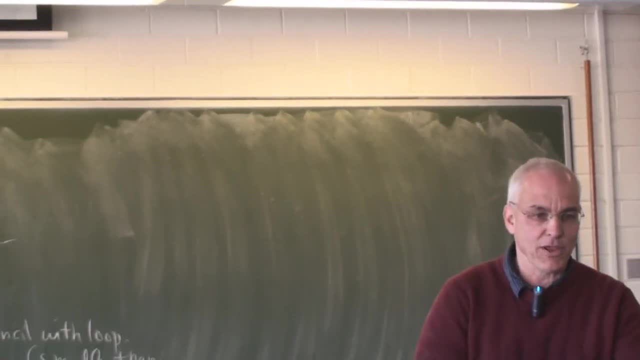 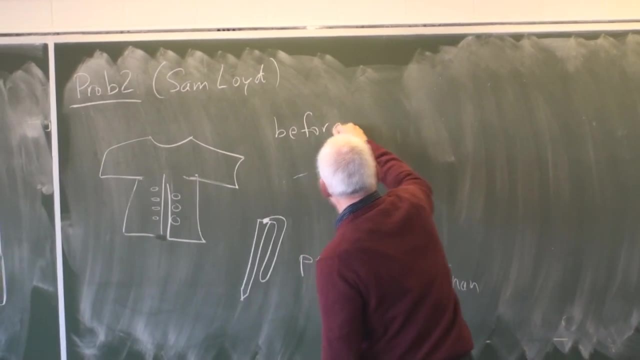 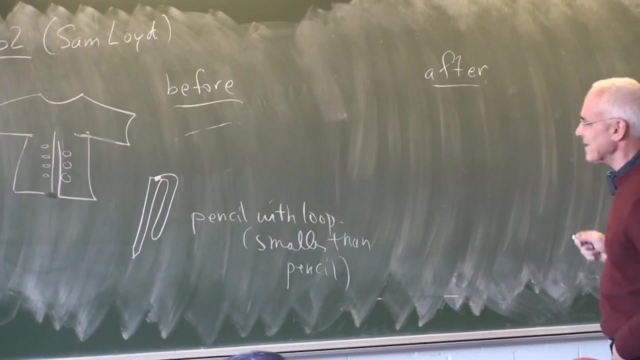 you can do it. You say: look the other way for a second and you do something quickly, And then afterwards- this is before and then after- you end up with something that looks like this: Okay, Okay, so here's our shirt. 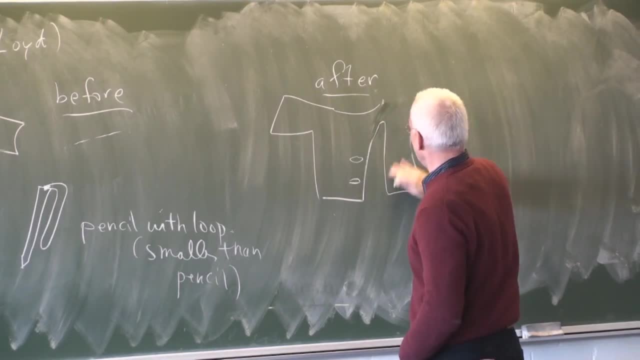 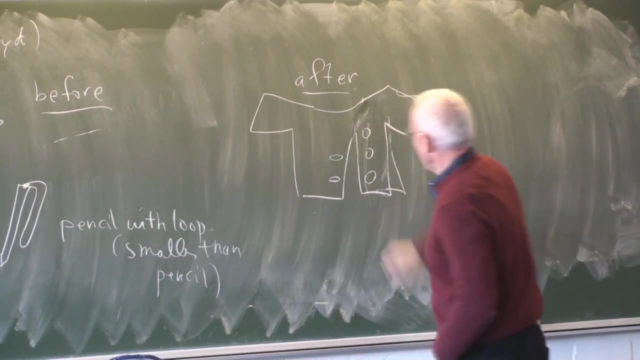 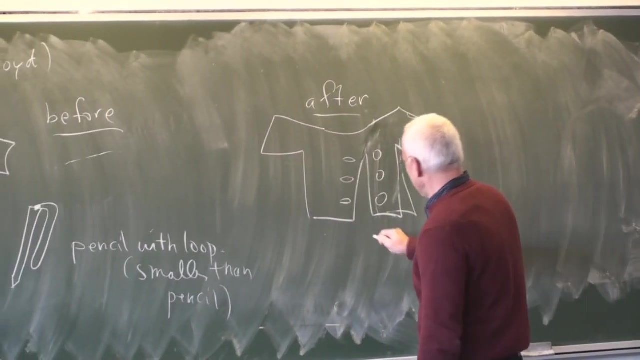 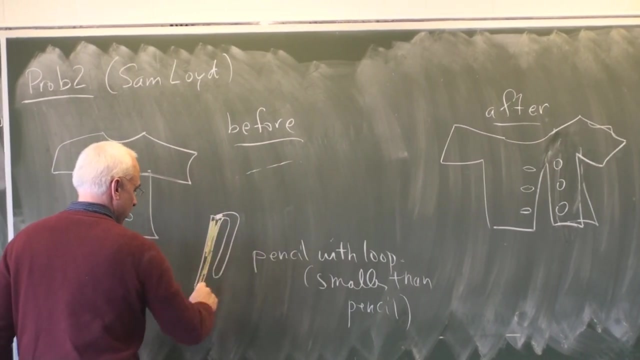 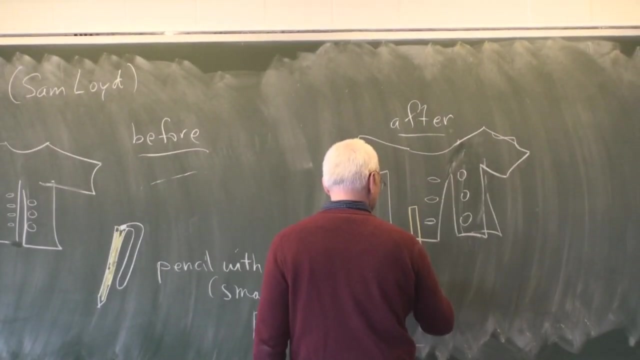 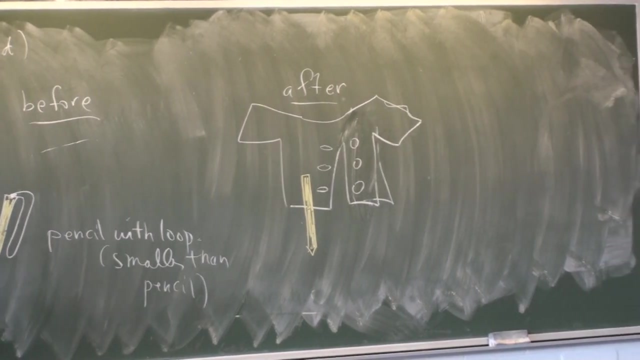 The button's there. Okay, so we've taken one of the holes, and what happens? I'll call this pencil yellow. Okay, so the pencil is now like this, And what about the loop? Well, maybe it'll be purple. 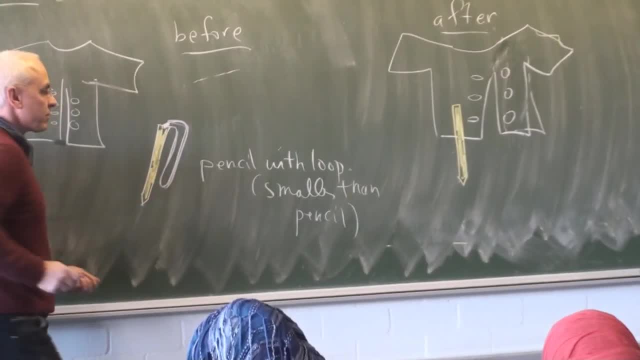 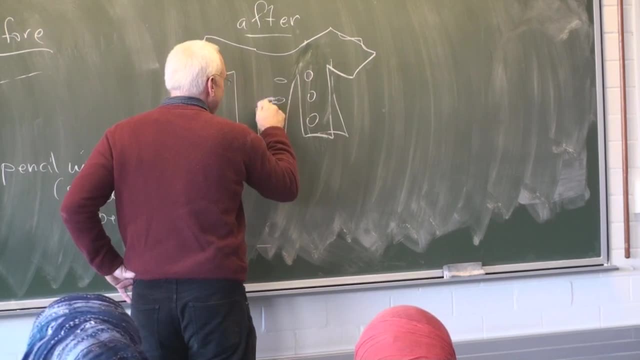 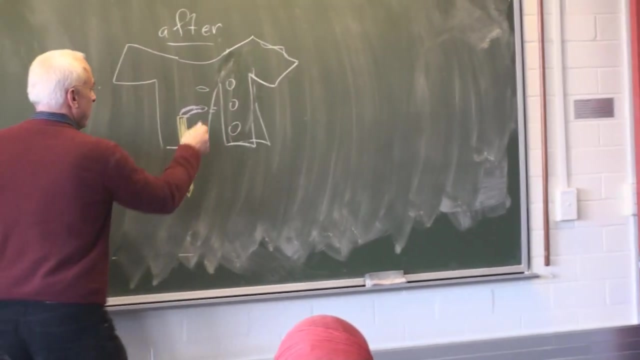 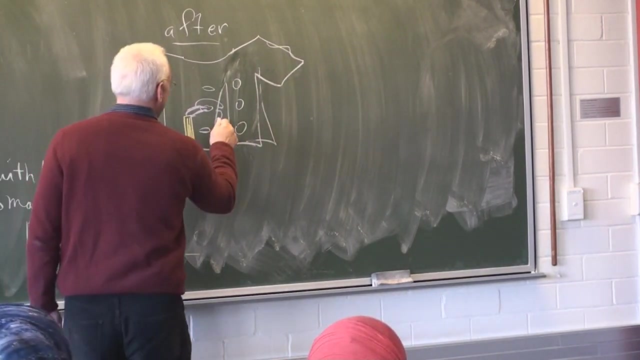 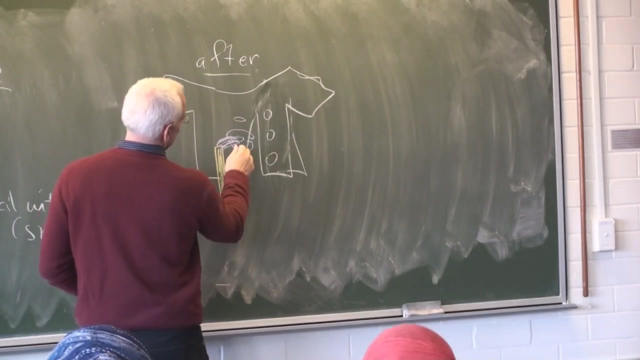 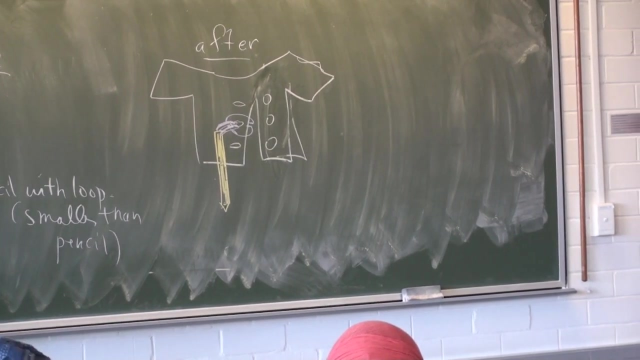 There's our purple loop. The loop looks like this: It goes through here, Then it comes out the back, It goes under, So it only uses one hole of the shirt. Yeah, it just uses one hole of the shirt. Okay, so the pencil is now attached to the shirt. 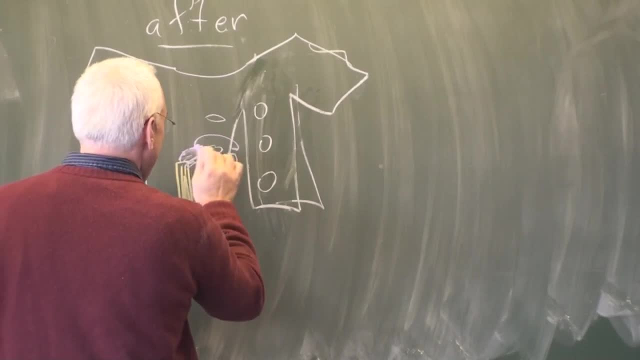 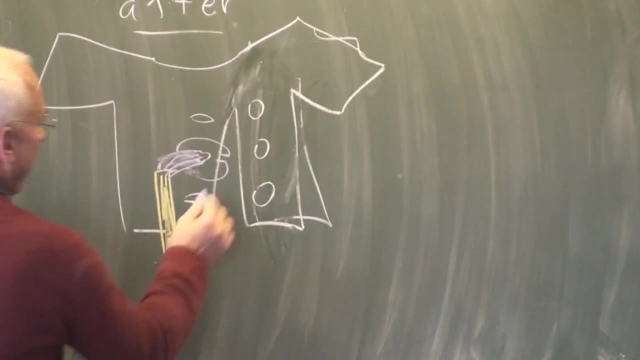 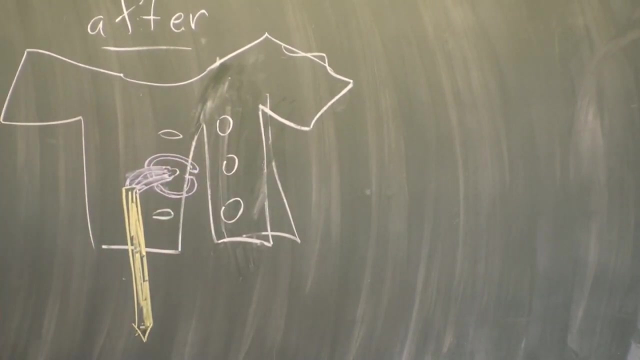 But this part goes over. Let me try to make that a little bit more clear. So there's that there And that goes into the hole, And then outside here. Oh yeah, we need to preserve holes. This is topology, Yeah right. 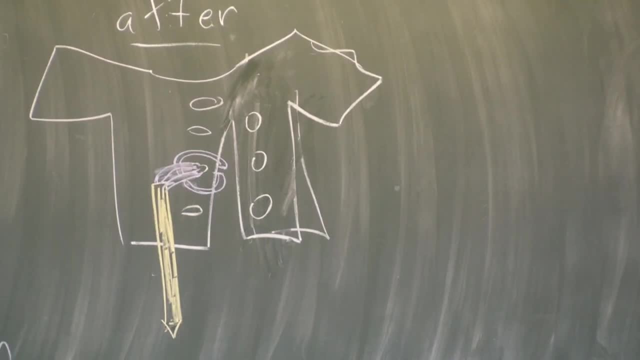 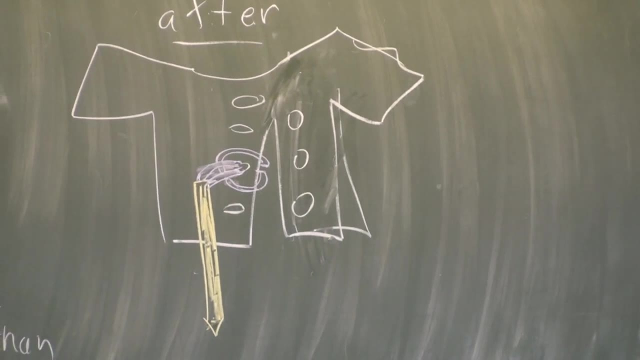 Okay, thank you. Okay, now, So is that? Is that a double piece of string everywhere? Huh, This is a solid piece of string. This is a solid piece of string. You draw it with double? Okay, I'll draw it. 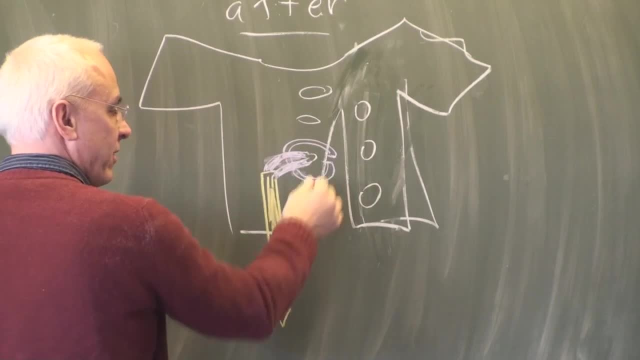 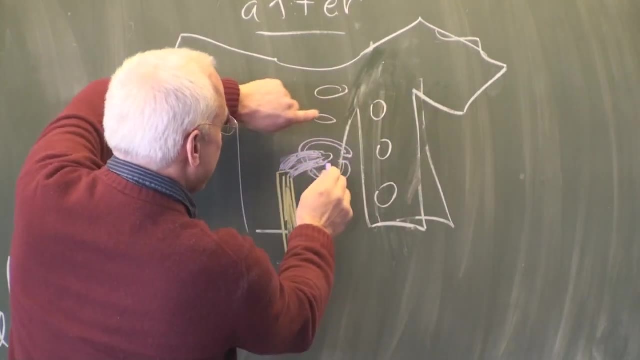 I'll just make it a little bit thicker. I want to make it clear that this is in front and that's behind. Oh, but that's So, it's all. So the thing goes in the hole, then comes out sort of dot dot dot through there. 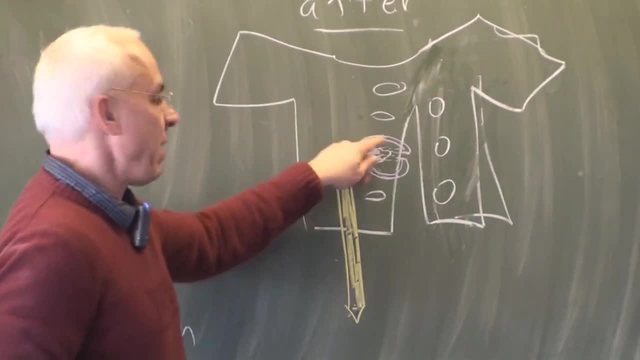 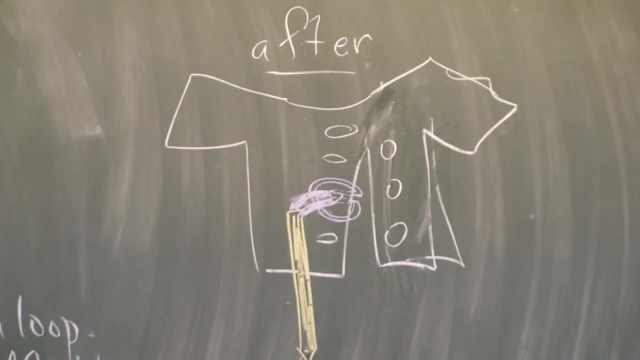 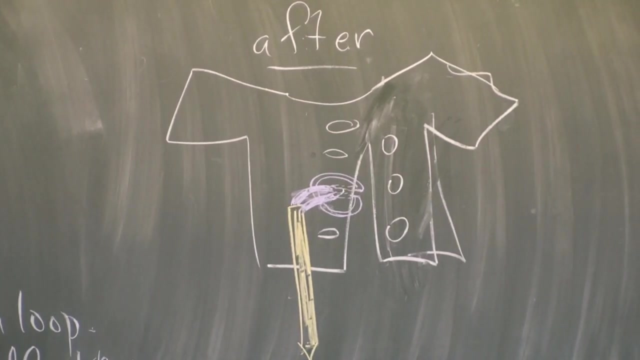 Then it comes out the back. If this was on top, you just pull the pencil out, Right, But it's looped under. so now the pencil is stuck. Do you agree? The pencil is stuck, And so the question is: 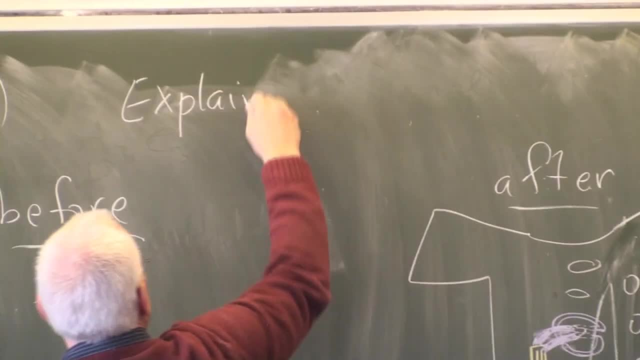 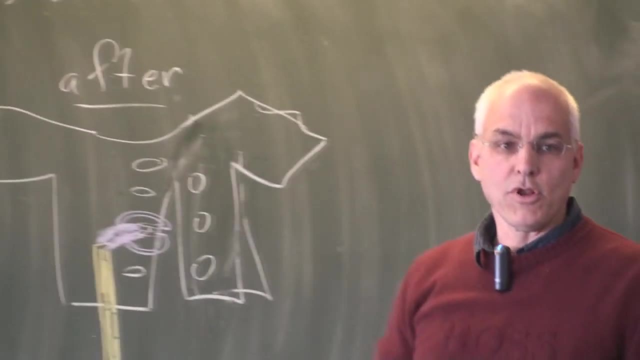 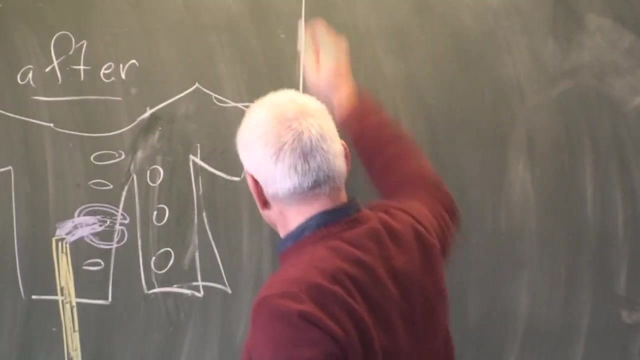 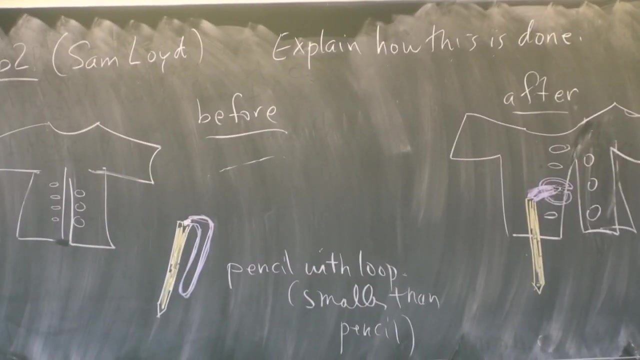 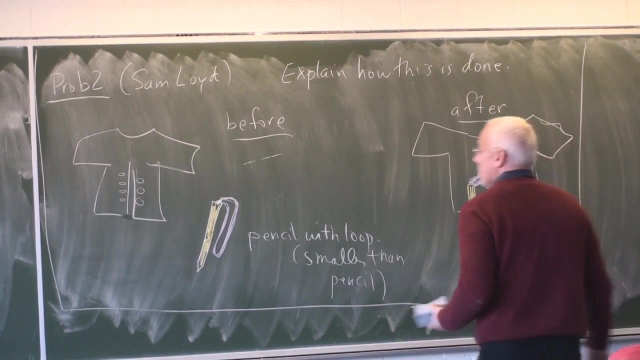 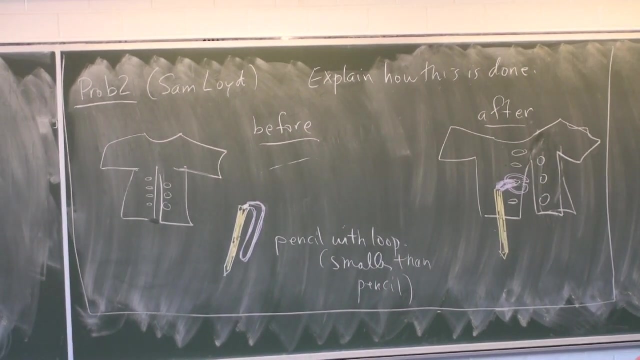 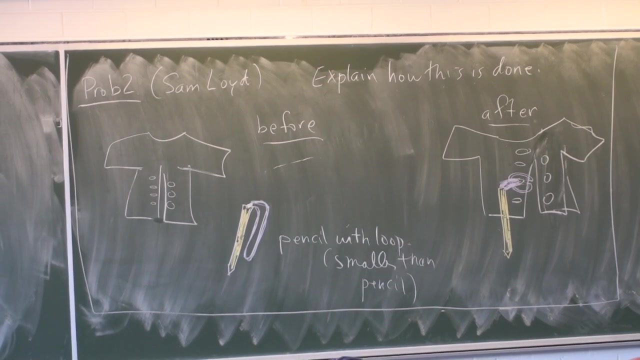 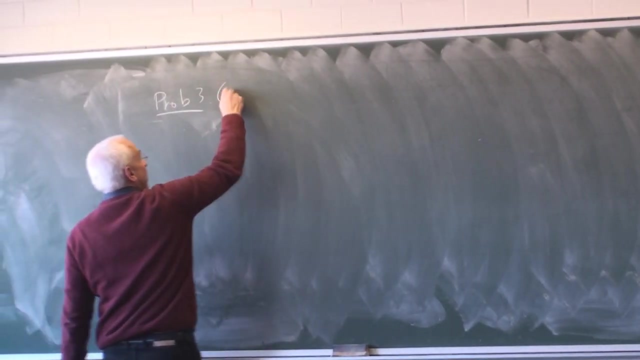 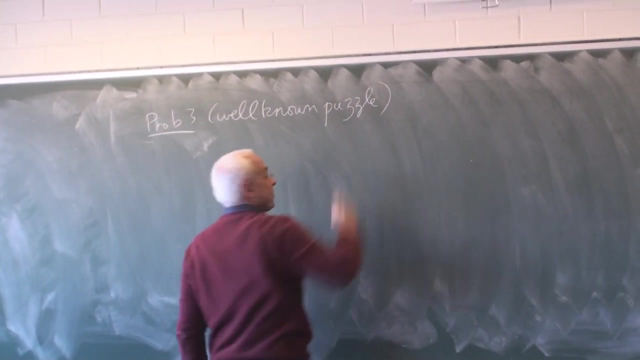 explain how this trick is done. You can also always make a model and try it out. It actually works, but you have to figure out how to do it. Okay, and problem number three. This is a well-known puzzle that you can find in many places. 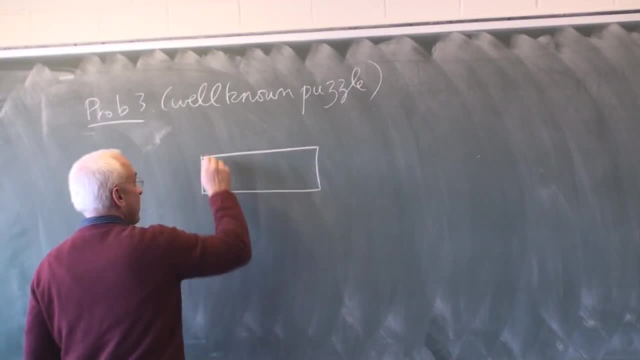 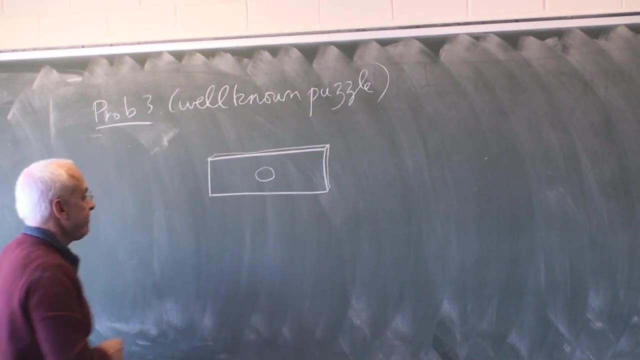 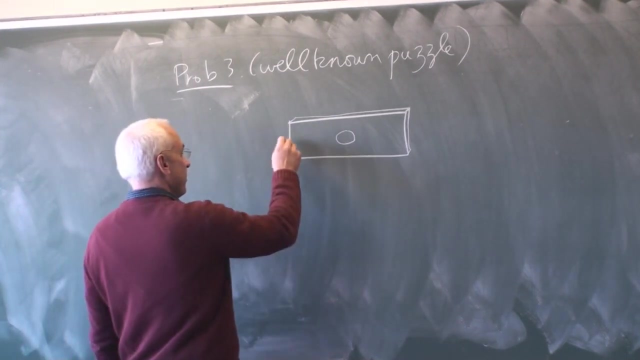 Okay, so we have a piece of wood. It's like a thin little piece of wood And it's got a hole in the middle And Okay, It's a lot like that. There's some string And the string comes up. 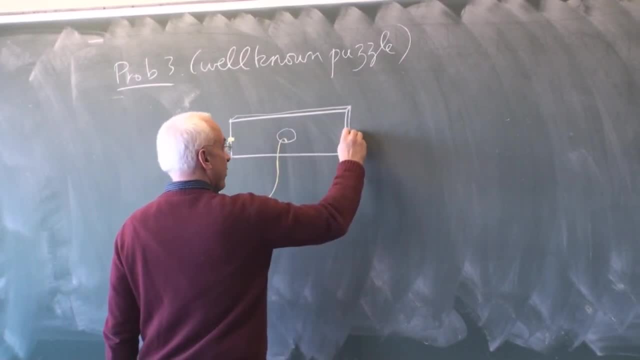 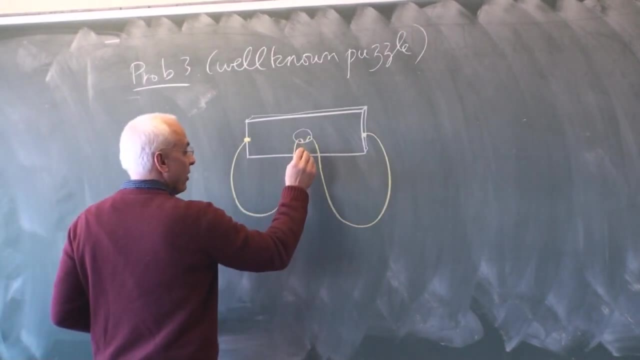 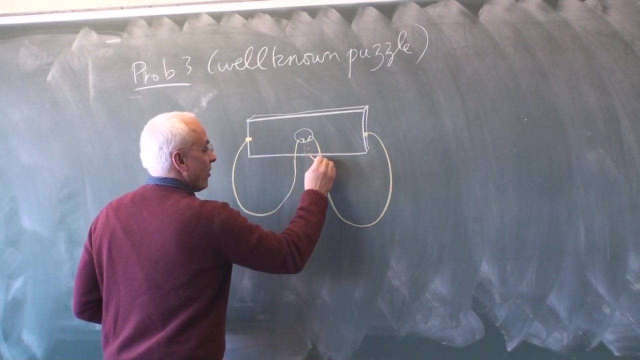 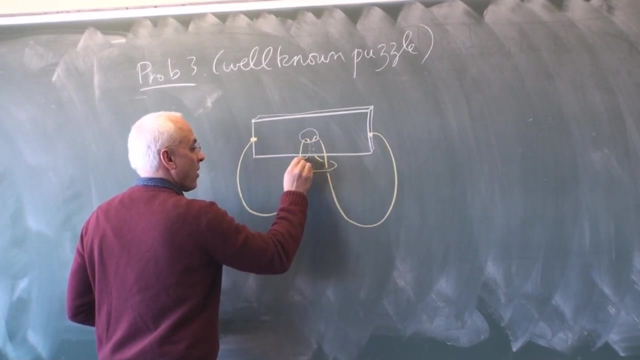 and through there And there's another piece that goes up and through there. It goes through the hole and comes out the other side And it wraps then around and through the other side And it wraps then around and through the other side And it wraps then around. 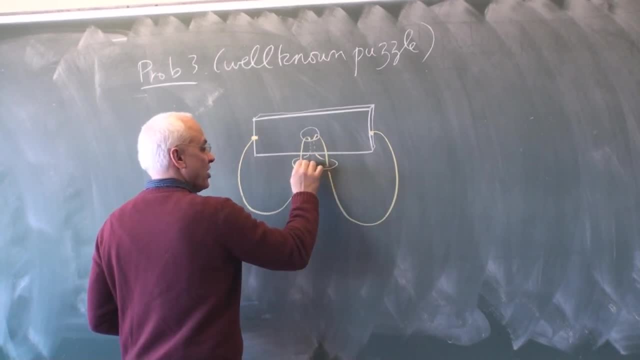 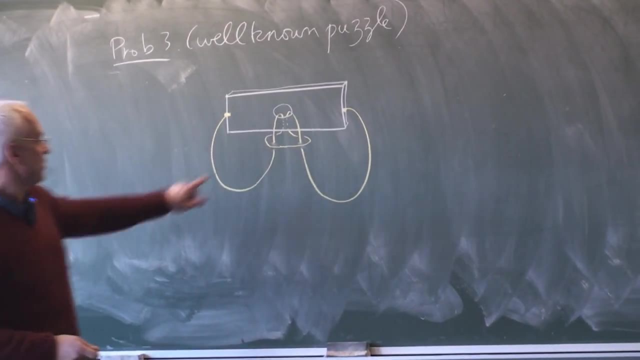 and through the other side. Okay, an advantage that I have with chalk is that it's easy to rub things off. It's just the nature of this topology. Okay, so now you can see that there's a. Yeah, it's a lot like the shape over there.